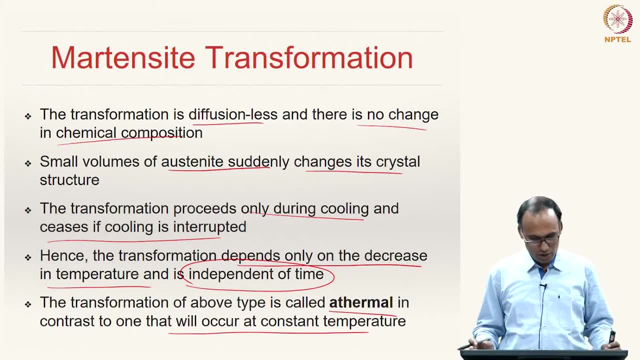 will transform to martensite. So we have stopped the discussion at this particular slide where we are discussing the transformation. martensite transformation- As we have already mentioned, the transformation of austenite to martensite is a diffusionless transformation and hence there is no change in chemical composition and the small volumes of austenite suddenly 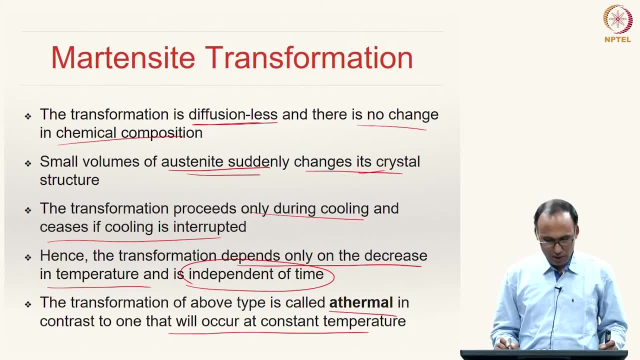 changes its crystal structure. when you are rapidly cooling the austenite, rapidly cooling the eutectoid alloy, The small volumes of austenite suddenly changes its crystal structure and thus transformation proceeds only during cooling and ceases if cooling is interrupted, That means if you 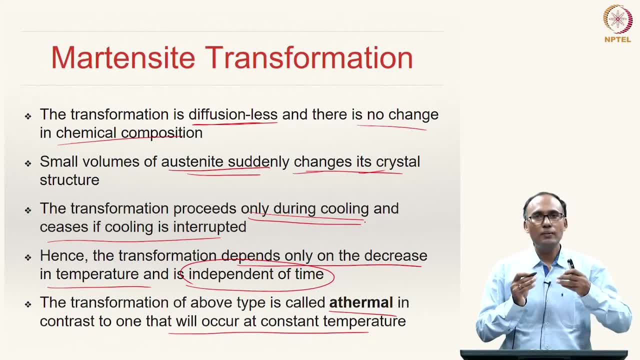 stop continuing to reduce the temperature beyond martensite- short temperature martensite. further reaction from austenite to martensite or further transformation of austenite to martensite will not happen. Hence the transformation depends only on the decrease in temperature. 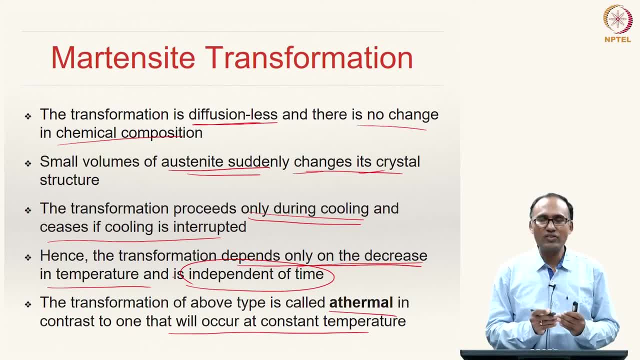 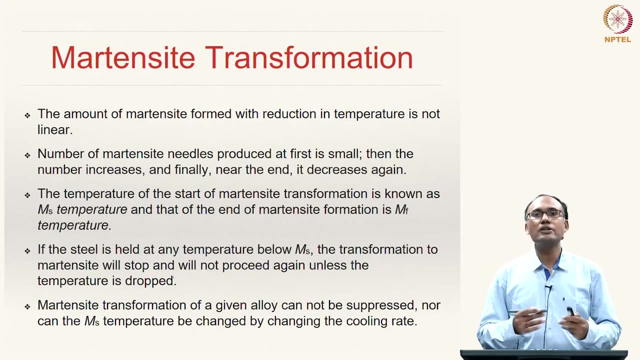 and is independent of time. So at a given temperature, even if you keep for sufficiently long time, however long you keep- that transformation will not happen, because it- the martensite transformation- is only a temperature dependent transformation. It always happens at a constant temperature and it happens readily. there is no time involved. 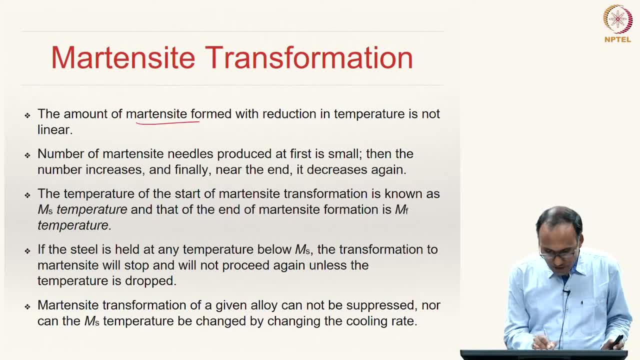 there, All right. So the amount of martensite transformed with reduction in temperature is not a linear function. That means if you are reducing the temperature from martensite, short temperature below the amount of the transformation from austenite, austenite to martensite does not scale linearly with the temperature reduction And the number. 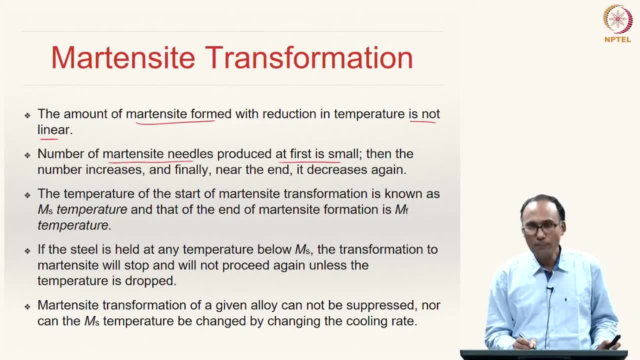 of martensite needles produced at first is small and then the number increases and finally, near the end it decreases. So it is like an S shaped curve where initially you have a small accumulation or small transformation, small amount of transformation of austenite. 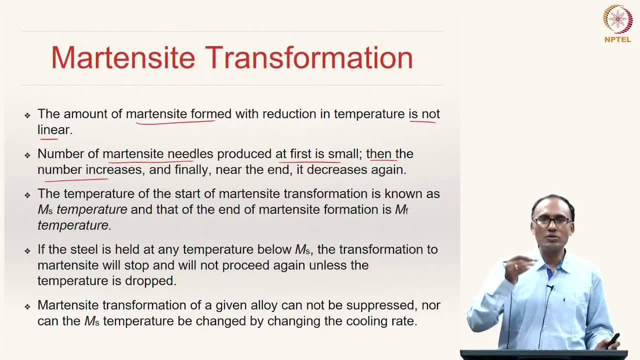 to martensite and in between. after that the transformation rate will be more. So that means at higher somewhere in between temperature. here when I say in between, it is not the time, but the temperature. right At a very close to martensite start temperature, you will. 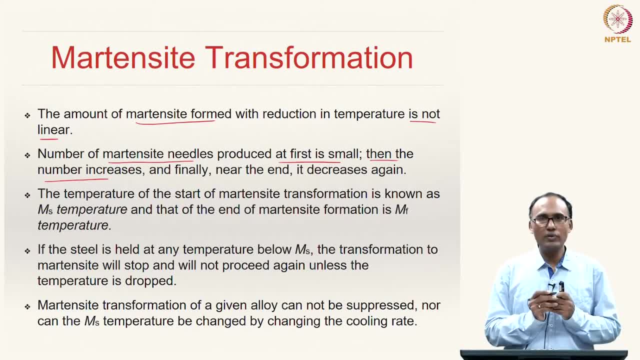 have the martensite needles produced at a very low and, as you are in the middle range of this martensite start to martensite finish temperature, then you will have reasonably steep increase in number of martensite needles and finally it decreases again. 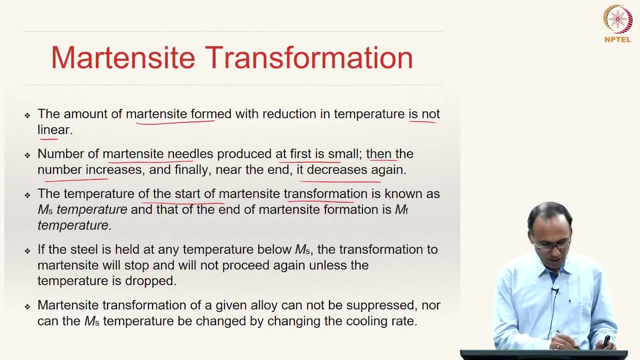 So the temperature of the start of martensite transformation is known as F, MS or martensite start temperature and the temperature at which martensite transformation finishes. that means, when austenite transforms to martensite completely, then it is called. 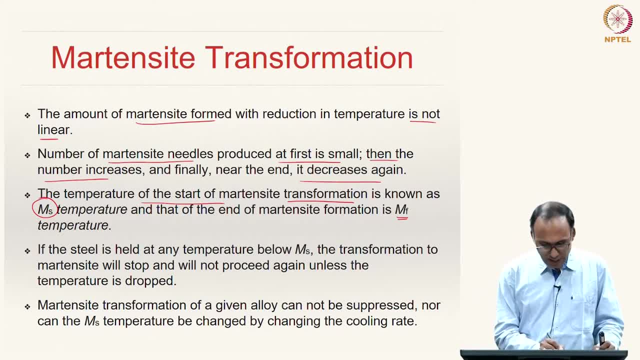 martensite finish temperature. If the steel is held at any temperature below MS then the transformation to martensite will stop if you are holding at that particular temperature and will not proceed unless the temperature is dropped, And so the martensite transformation. 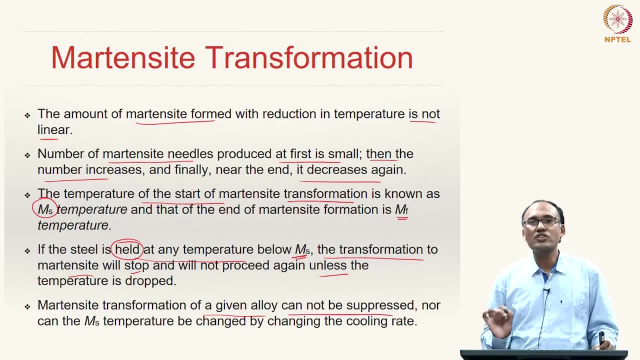 of a given alloy usually cannot be suppressed. If you are doing it a very fast, if you are cooling the alloy at a very high rate of cooling, if you are heating the martensite start temperature, it will transform from austenite to martensite. 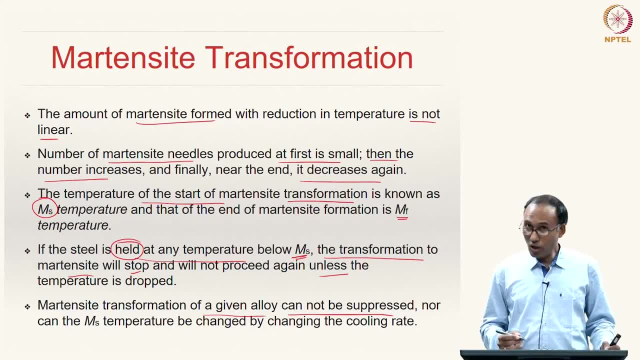 right. So there is no way that we can suppress this, And nor the MS temperature. the martensite start temperature also cannot be changed by the cooling rate. It only depends on the alloy composition. For a given alloy composition, martensite start temperature is fixed. So 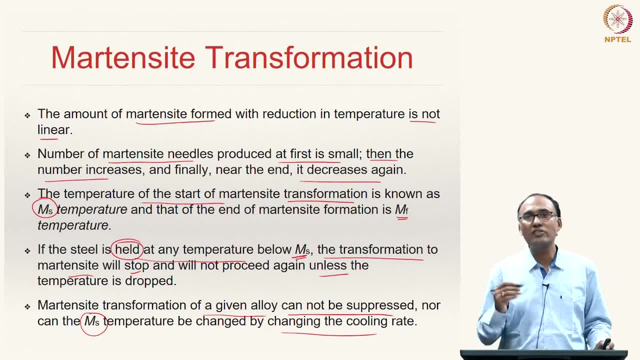 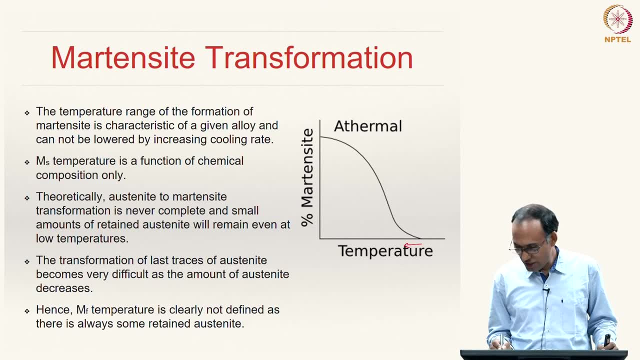 as you are holding the soil, había kerasas and the martensite finish temperature is fixed. you cannot change those temperatures for a given alloy. All right, So, as you have seen, as you are reducing the temperature as you are initially, 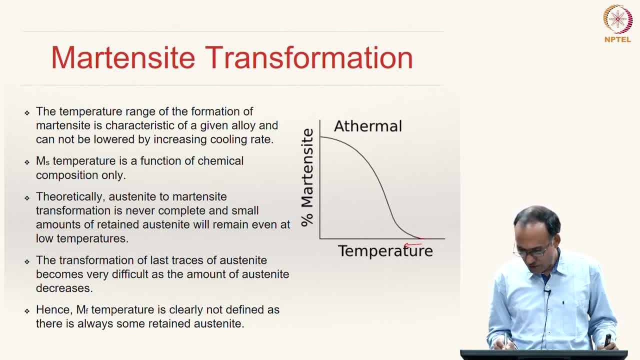 the martensite transformation will be less And, as you are, or during further reducing the temperature, the martensite transformation picks up and again in the end it slows down. So the temperature range of the formation of martensite… so that is martensite start. 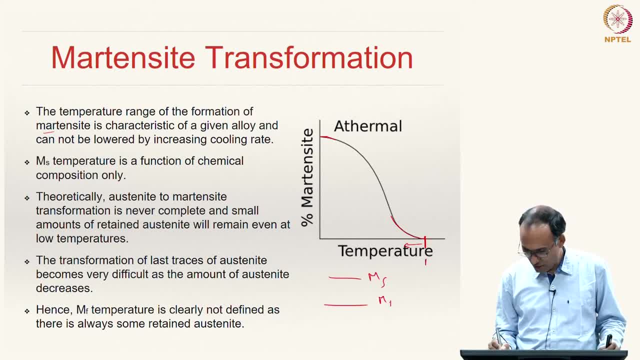 temperature to martensite finish temperature. So this is sort of your martensite start temperature temperature and this is probably martensite finish temperature. So this range during which the martensite transformation happens from austenite is a characteristic of a given 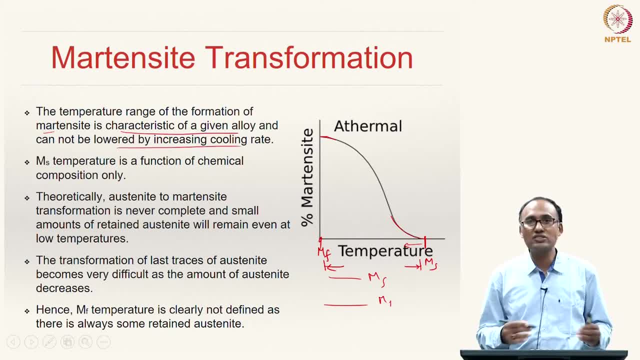 alloy and cannot be lowered by increasing the cooling rate. So it does not depend on the cooling rate and, as we have already mentioned, M S temperature is a function of chemical composition only. So if you are taking about 1 0 8 0 steel and 1 0 9 0 steel, their martensite. 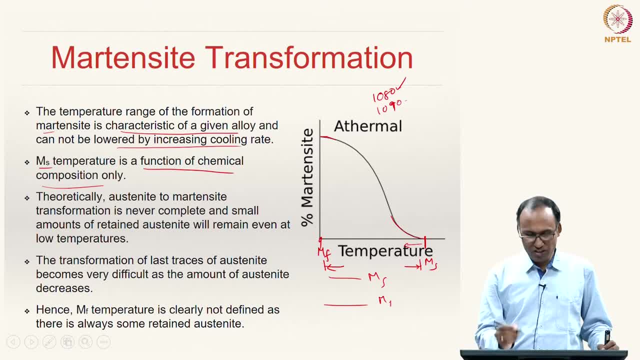 start temperature and finish temperatures is fixed. this one will have specific martensite start temperature. this one will have an specific martensite start temperature. So martensite start temperature depends only on the chemical composition, not on the cooling rate. So theoretically, the austenite to martensite transformation is never complete. That means 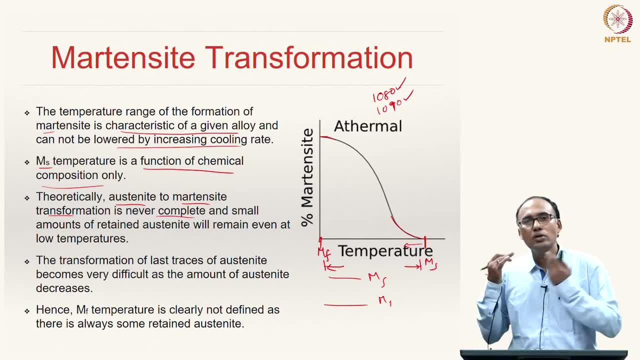 you will not have 100 percent martensite transforming to sorry, 100 percent austenite transforming to martensite. So theoretically it is never complete and small amounts of retained a austenite austenite will remain even at low temperatures. some amount of So whenever we are saying 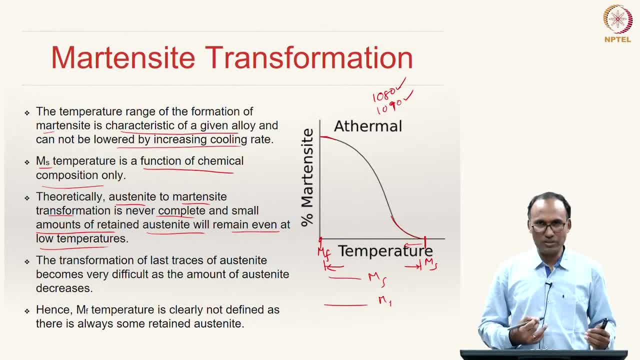 that martensite finish. it is not necessarily 100 percent, probably 99 percent. So remaining 1 percent austenite is retained as retained austenite. So the transformation of lost traces of austenite becomes very difficult as the amount of austenite decreases. Hence 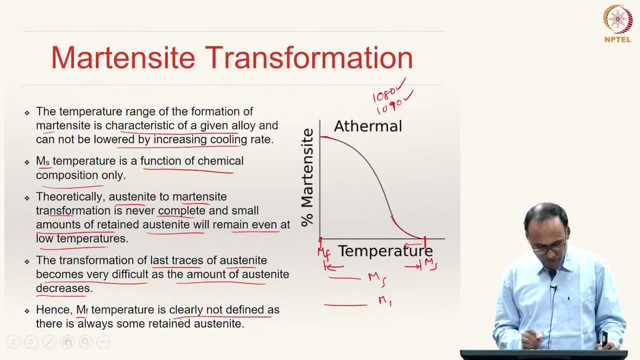 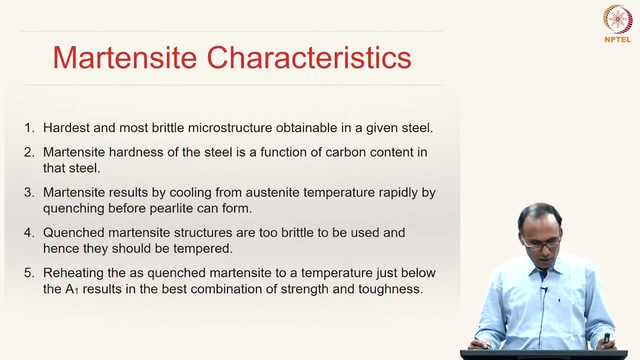 the M F temperature. the martensite finish temperature is clearly not defined as there is always some retained austenite in the product. So the martensite is the hardest and most brittle microstructure that is obtainable in a given steel For a given alloy. composition of iron and carbon for a given steel alloy. 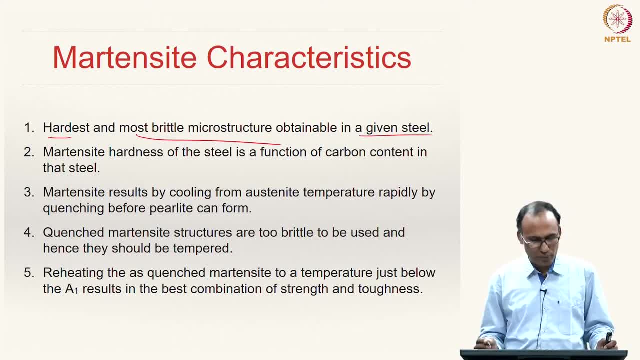 the martensite microstructure is the hardest and brittle microstructure that one can obtain, And the martensite hardness of steel is a function of carbon content in the steel. We know that the as you increase the carbon content, you will increase the hardness and brittleness Similarly. 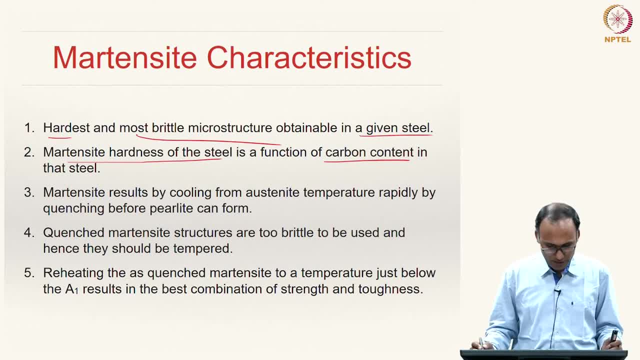 the martensite hardness. amount of hardness is also a function of carbon content. So the martensite results by cooling from austenite temperature rapidly by quenching before pearlite can form. So how do you get it? So you actually, before the pearlite can form, you quench it. 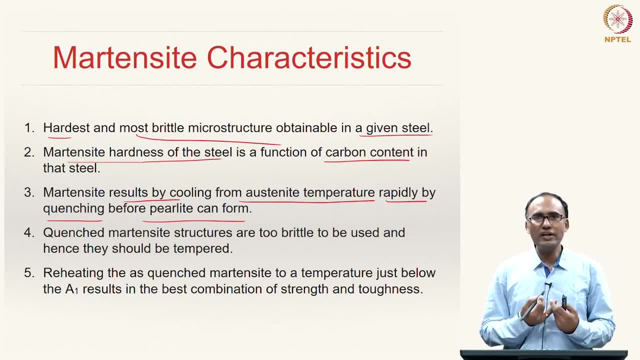 So that quenching means rapid cooling. You rapidly cool austenite such that no pearlite is formed. So all the way you bring the temperature down to martensite start temperature and that is when your austenite transforms to martensite. So the quenched martensite structures are. 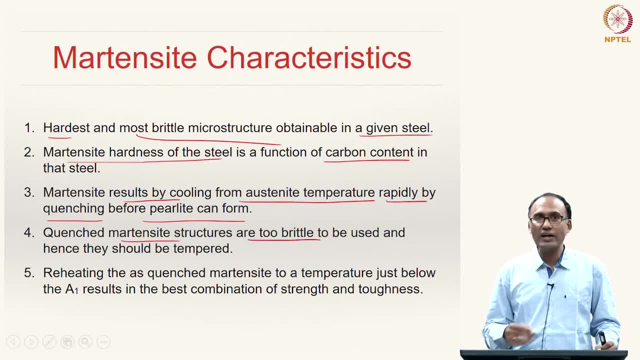 too brittle. because of the rapid cooling rate and the microstructure development, They are known to be extremely brittle And hence they cannot be used for applications right away unless they are tempered, So they should be undergoing all the martensitic microstructure. 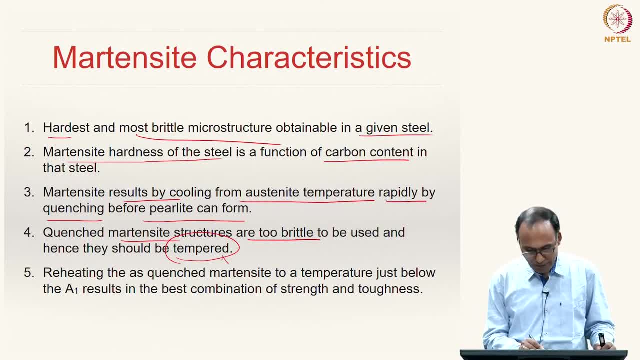 should be undergoing. This is a heat treatment process called tempering. Only the tempered martensite will offer some additional strength and toughness. Otherwise, in its quenched form, martensite is extremely brittle to be used for any technological applications. So reheating the as quenched martensite to 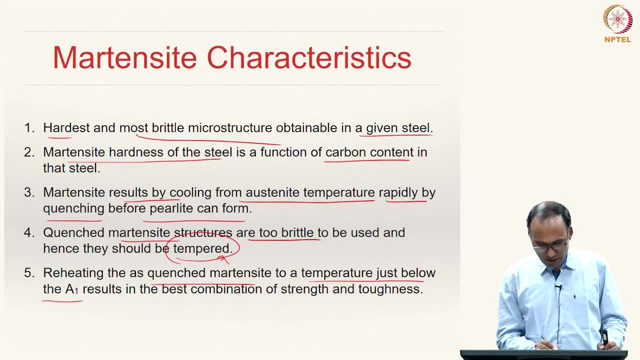 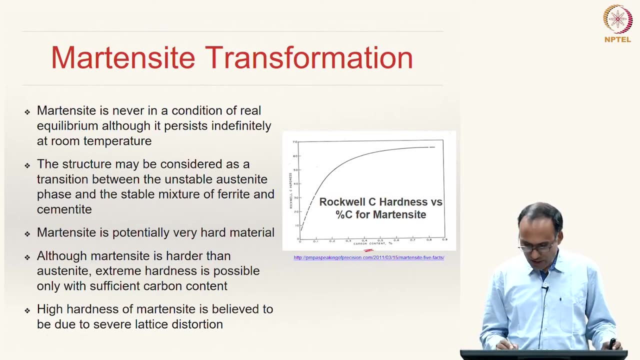 a temperature just below A 1, that means lower critical temperature results in the best combination of strength and toughness. So you need to do another heat treatment process after obtaining quenched martensite. So in that sense the structure, the martensite structure, can be considered as a transition. 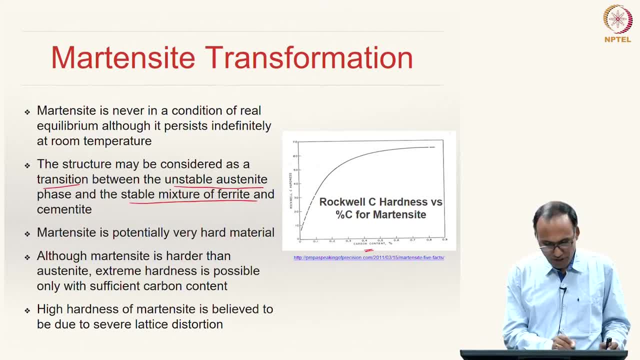 between unstable austenite phase and stable mixture of ferrite and cementite. It is a some phase in between unstable austenite and a stable perlite microstructure And, as we have discussed, it is potentially very hard material, Although martensite is harder than. 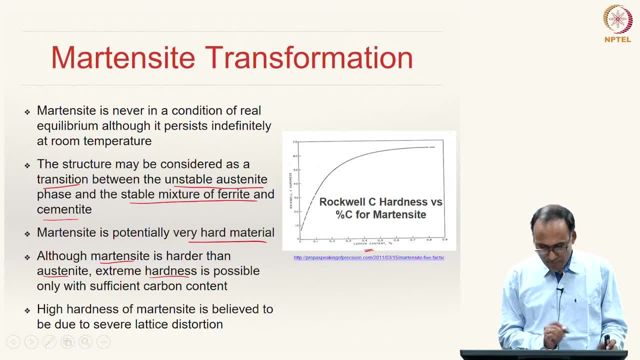 austenite, extreme hardness is possible only with suffocation. So it is possible only with sufficient carbon content. If you do not have enough carbon content, you may not have good enough hardness. So and another reason why the martensite shows extreme hardness. 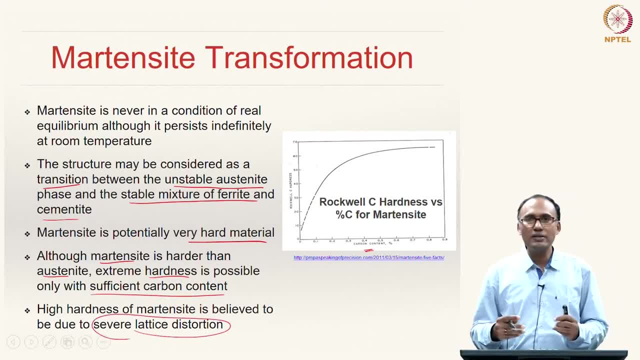 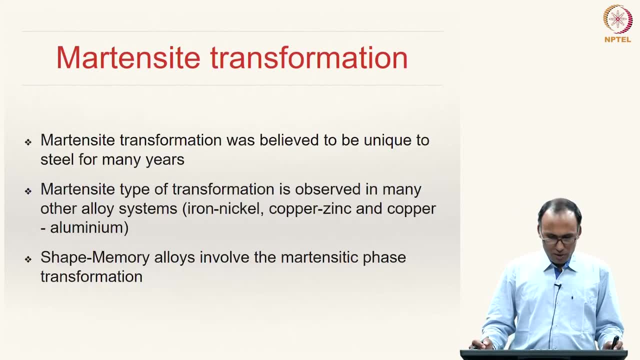 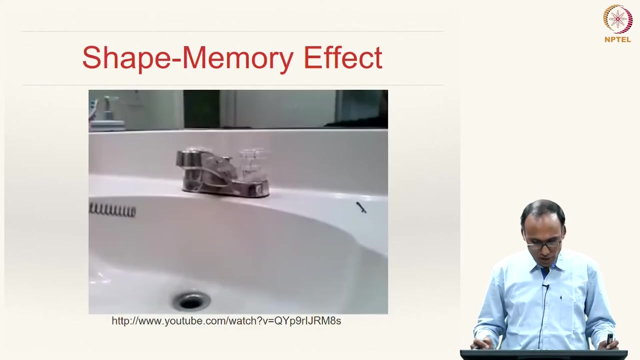 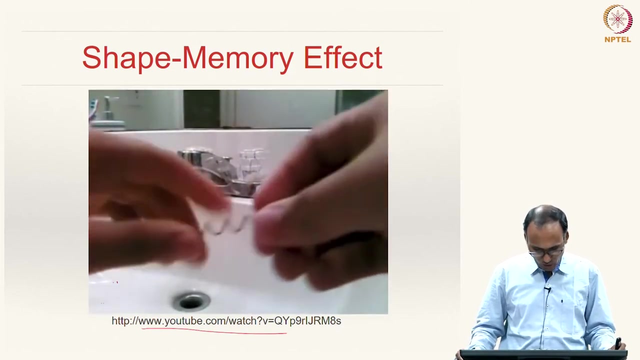 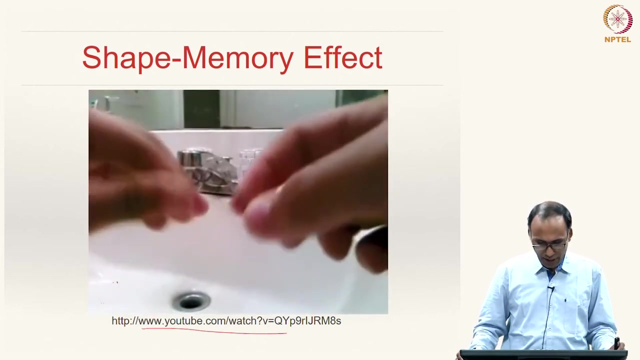 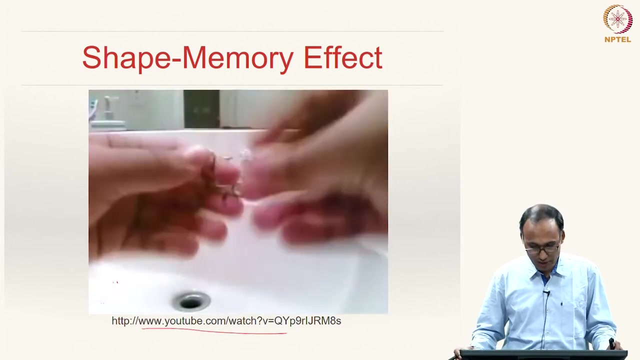 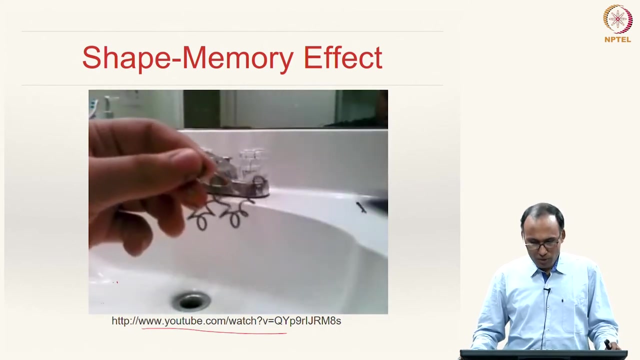 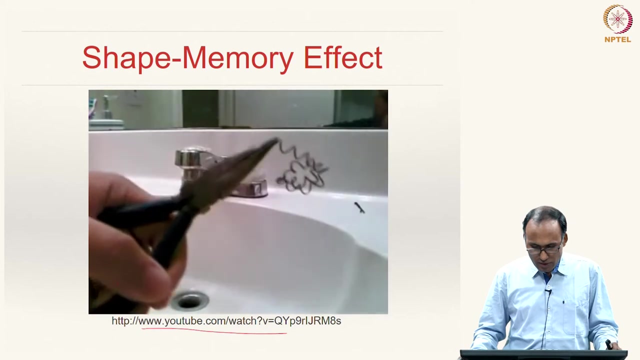 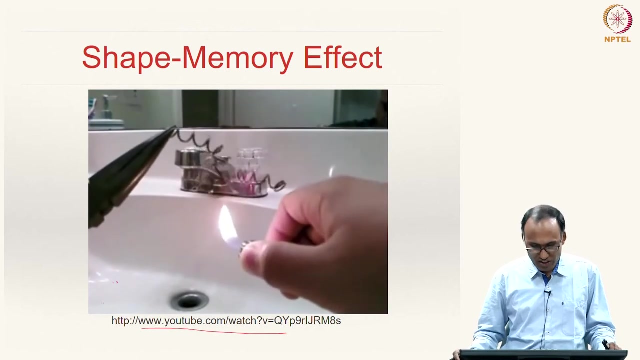 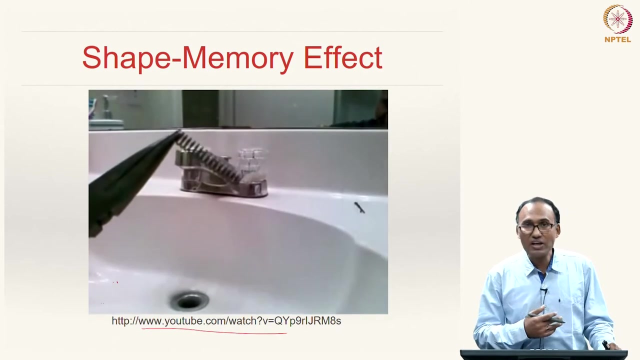 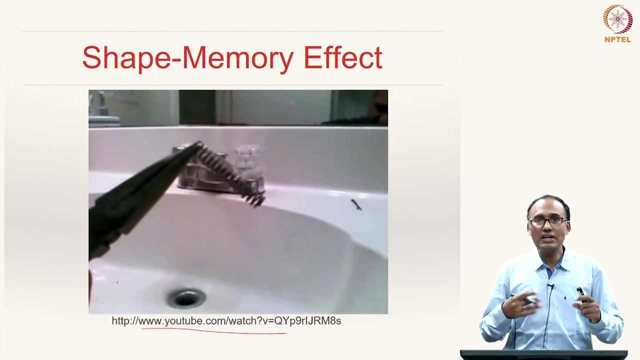 is because of the severe lattice distortion that is caused by the trapped carbon atoms in the lattice. So typically so people. when we were, they were studying about martensite- transformation of austenite to martensite. I encourage you to go through certain literature that is available on shape memory effect in 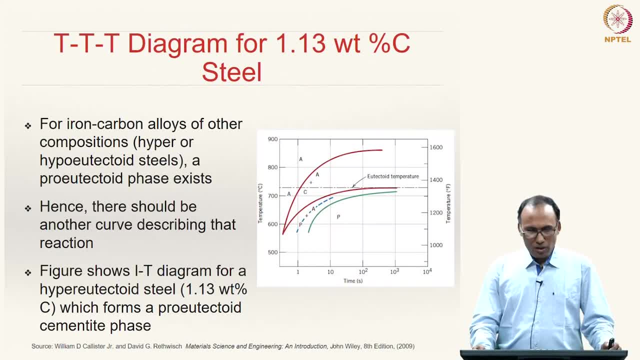 several text books or the online resources. So now we have seen the time temperature transformation diagram, or isothermal transformation diagram, for a eutectoid steel. However, how does such a time temperature transformation diagram looks like for a non-eutectoid? 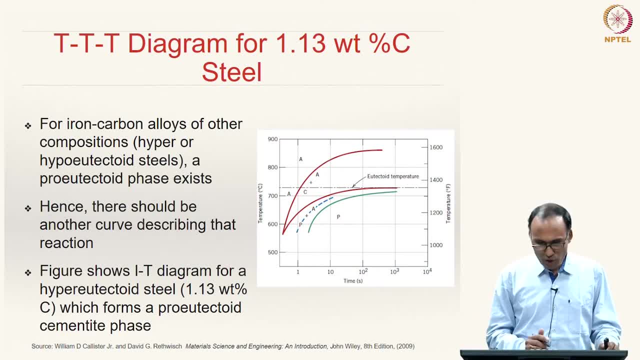 steel, either hyper eutectoid steel or a hypo eutectoid steel. Here we are showing the TTT diagram for 1.13 percent weight percent carbon steel, which is a hyper eutectoid steel. So when we are cooling down this guy, the microstructure that we would expect from our 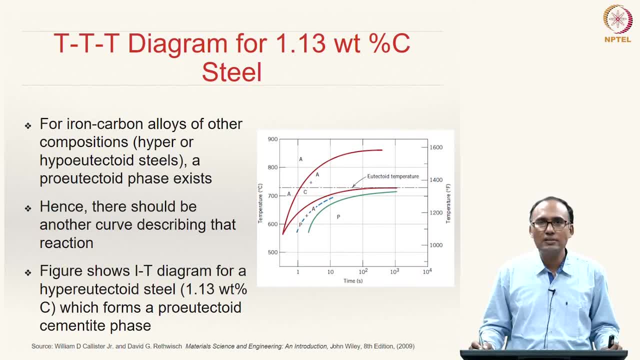 study on phase diagrams is that you will have a pro? eutectoid cementite. So austenite first transforms to pro eutectoid cementite above the lower critical temperature A 1, and once it touches A 1 then it starts transforming to eutectoid mixture of ferrite. 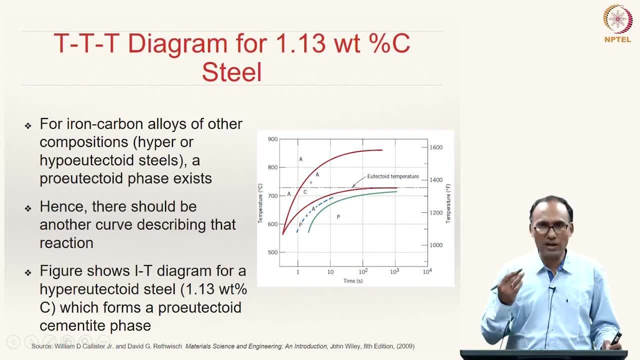 and cementite. So you have a pro eutectoid cementite phase and a pearlite phase. So you can clearly see, here you have an additional curve which basically represents your pro eutectoid cementite phase. So if you are at eutectoid temperature and above that, you will have transformation to 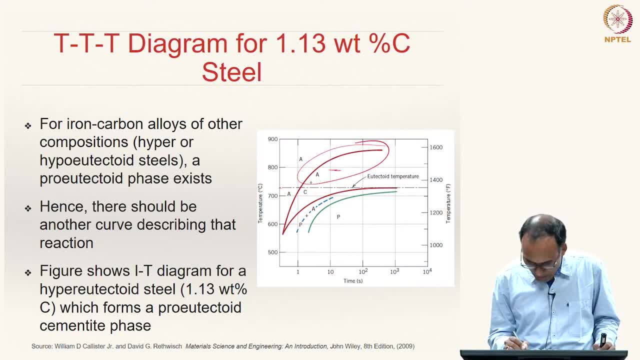 pro eutectoid cementite phase. so that is why this region is A plus C. that is cementite, and once you are below the eutectoid temperature then you will have transformation from the remaining austenite- whatever austenite is remaining. 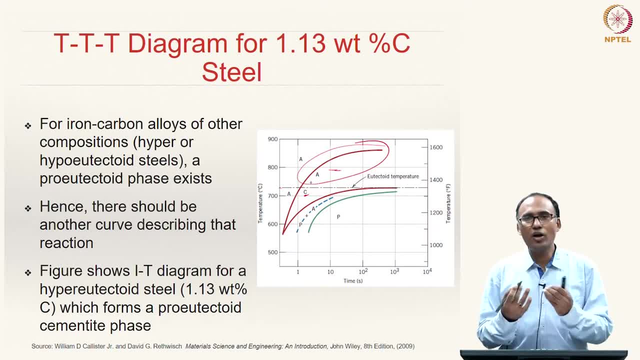 So some amount of austenite is transformed to eutectoid, So agent is transferred to cementite and remaining austenite would transform to eutectoid mixture of pearlite, So ferrite and cementite that is pearlite. so that is what is basically, if you are cooling. 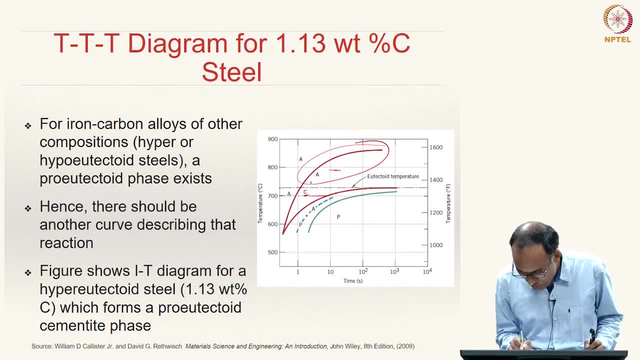 down to 700 degree Celsius. Then you are waiting here and then you see that between point A 1 and A 2 you will have austenite A 1 to A 2, austenite transforming to cementite Right. 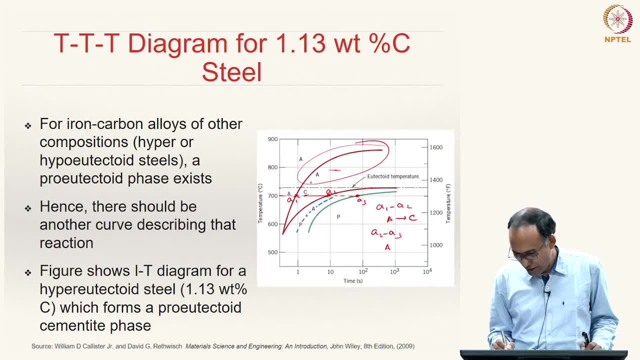 and A 3, A 2 to A 3, austenite transforms to pearlite And at the after A 3, you will have the microstructure has pro eutectoid cementite plus pearlite right. So you can see this. 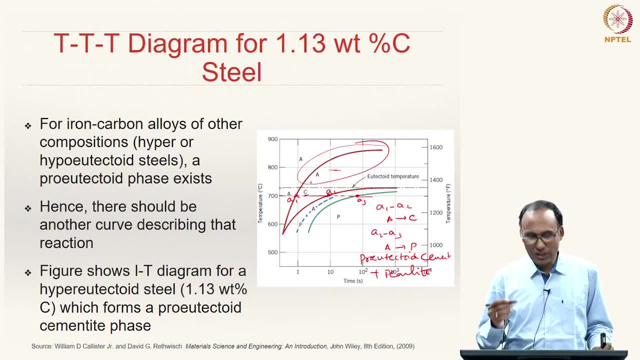 additional curve represents this pro eutectoid transformation, as we have already discussed. And here what you will know is how much time does it take for austenite to transform for a given alloy? for this is 1.13 weight percent carbon. So you can see that if you rapidly 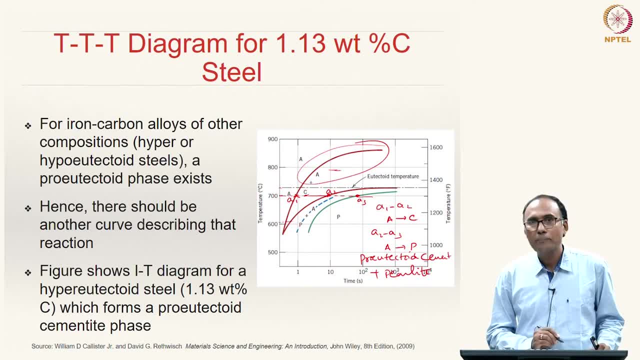 cool it down, the amount of pro eutectoid phase reduces. you can see that right. So here, at higher temperature, the amount of pro eutectoid phase is more, and at lower temperature, the pro eutectoid phase, the pro eutectoid fraction of pro eutectoid phase, is going to be less. 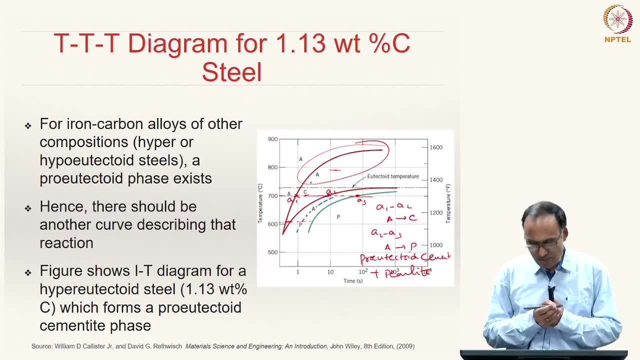 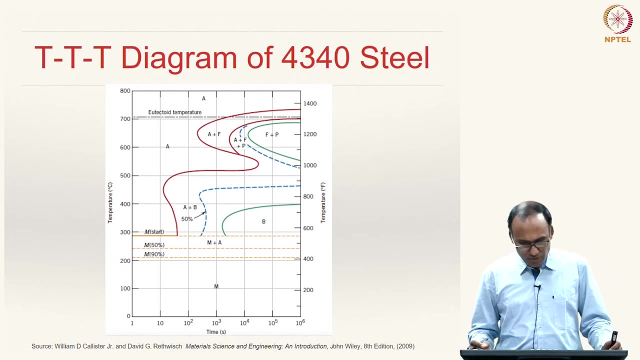 and most of it will be converted to pearlite. So by the looking at this, you can actually design your cooling cycle in such a way that you can get the amount of cementite pro eutectoid cementite that you want in the microstructure right. So this way, this is a phase, the time 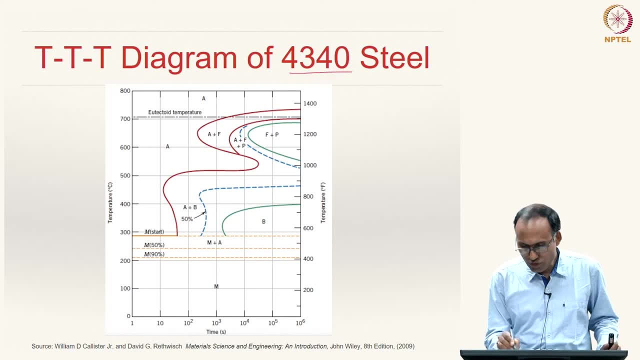 temperature transformation diagram for an alloy steel: 4, 3, 4, 0 steel right. So here 4 represents the type of alloy. what type of an alloy steel is this? and 3 is the 3 percent of that particular Predominant alloying composition. and 4, 4, 4, 0 represent 0.4 percent carbon right. So 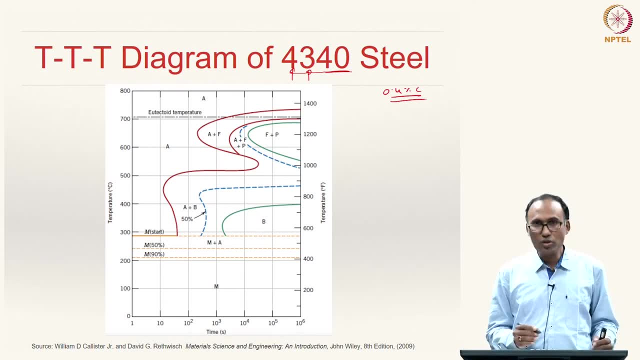 for this particular guy. you see that the time temperature transformation diagram looks much more complicated, right? So here you have austenite. here, because it is 0.4 percent carbon, you will have pro eutectoid ferrite phase, So that is why you have austenite plus ferrite. 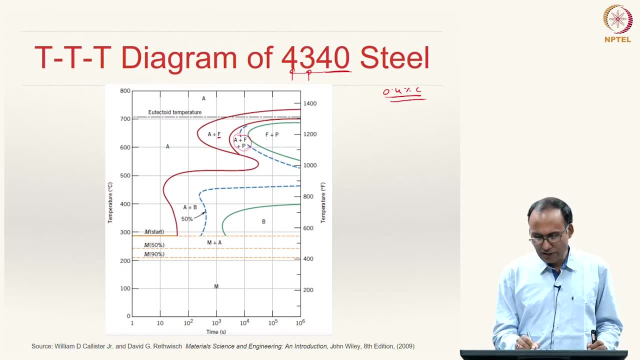 and then you will have austenite phase ferrite plus pearlite and then ferrite plus pearlite. right, Ferrite plus pearlite is because pro eutectoid ferrite and remaining ferrite. So you can see that Right. 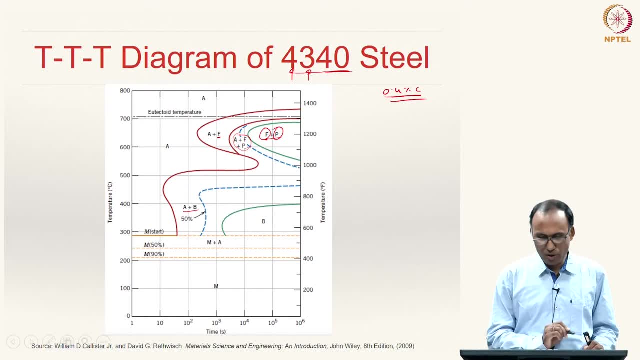 Remaining is pearlite and here you will see that bainite austenite is transforming to bainite below the nose right. This is a little bit more complicated t t t diagram, but not less. you will have again. there is martensite start temperature: 50 percent martensite transformation. 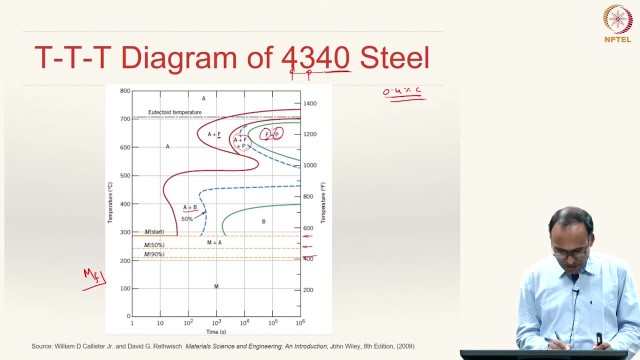 90 percent here. nowhere we have shown seen mf because, as we have discussed, martensite finish temperature line is very difficult to identify Because always there is going to be some amount of austenite that is going to be retained, So there will not be 100. 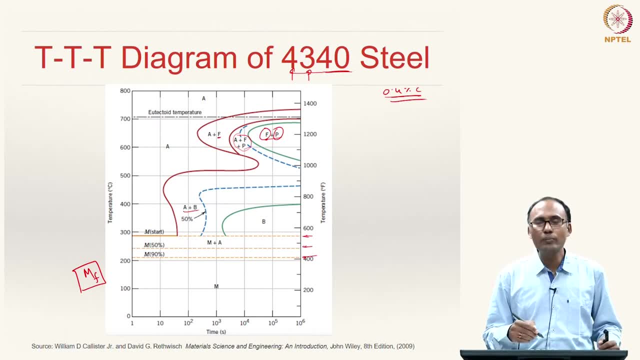 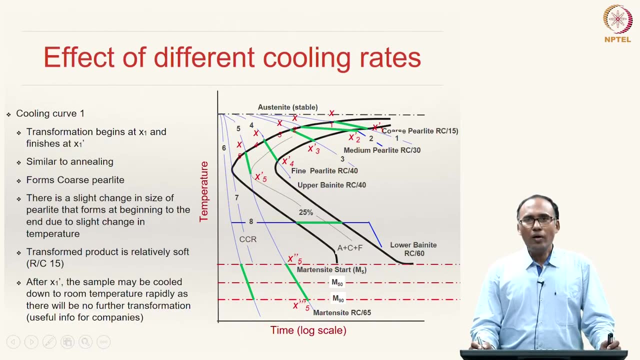 percent martensite line it is very difficult to identify. OK, When you lift up the iron, identify such lines. So usually most of the T-T-T diagrams will show martensite 90 percent. So now let us look at effect of different cooling rates and the resultant microstructures. 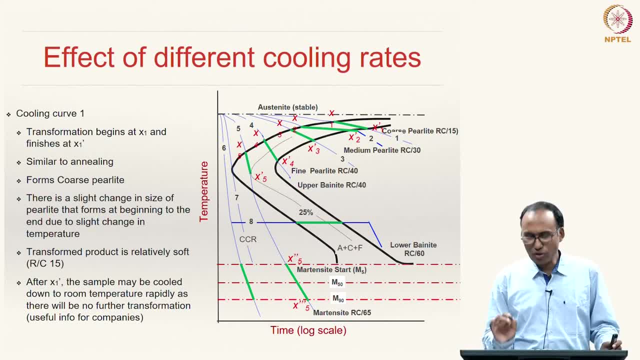 of the eutectoid alloys. We are paying attention to eutectoid alloys, So that is 0.8 percent carbon. So here we have 8 different cooling curves and we will see what sort of a microstructure one would get for each of these cooling curves. So here this is cooling curve 1, and from: 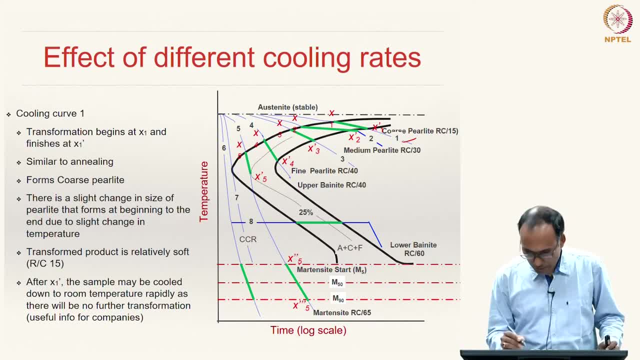 cooling curve 1 to 8, we have increase in cooling rate and my apologies for this. So this here: this is x 1 x, subscript 1.. So it got messed up and, because of the version, change from power point. So this is x 1, x, 2, x, 3, x, 4, x, 5 and so on, and this is your x 6 and this is your say. 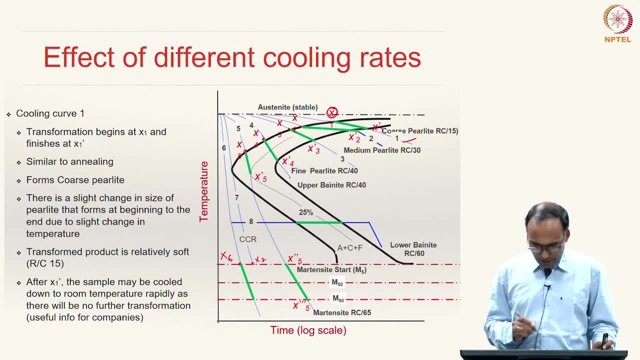 x 7- right, all right. So let us look at what is going to happen in this system. So, for instance, let us look at cooling curve 1- right, that is this guy and we have shown in between, on that line we have shown a green hatched line. that green hatched line represents the 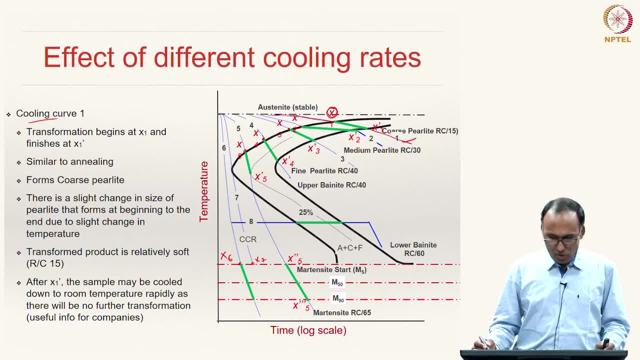 transformation progress scenario: right, So here you can see that, as you are reducing the temperature, So here x 1 is very slow cooling rate and you can see that the transformation begins until transformation does not begin until the time x 1, corresponding to x 1, reaches. 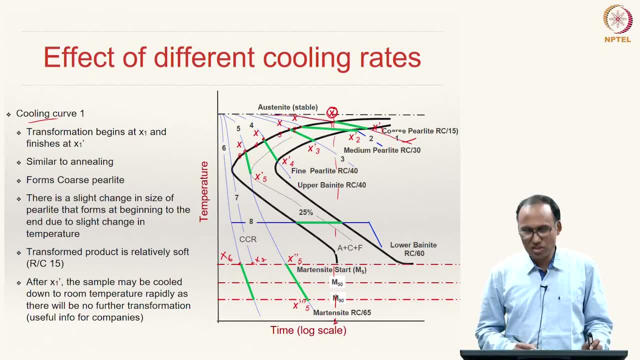 So until this time the transformation does not start. So, and then the transformation begins with: transformation begins at x 1 and cent ends at x 1 dash. and we can see that here we have: the transformation is happening at very high temperature, And at high temperatures the nucleation rate is low, but the diffusion 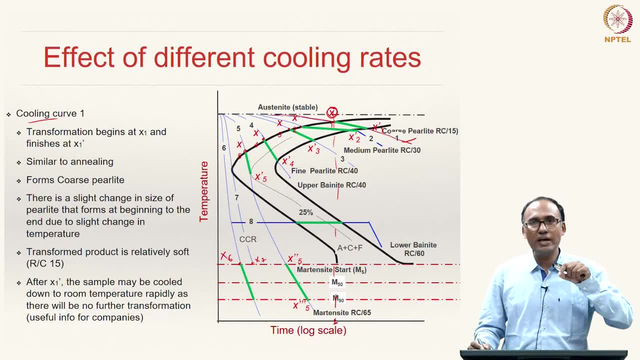 rate is high. So since the nucleation rate is low, the number of nuclei formed that few. and, as I reserved the microstructure, will be a course. so the end product here is going to be, course, pearlite. And besides each and every microstructure, we have also written the hardness, Rockwell. 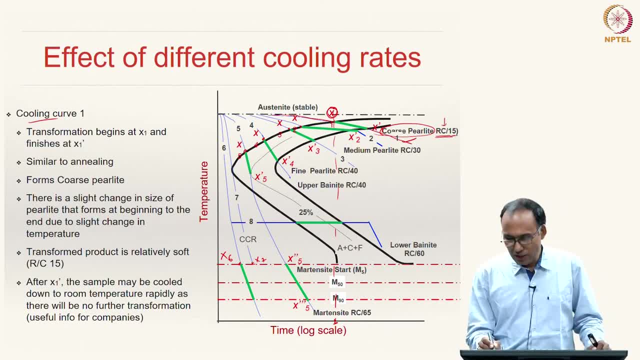 hardness on Rockwell scale C. Here you can see that here Rockwell hardness 15.. And as you are coming down the hardness increases. because you are increasing the cooling rate, the hardness also increases. So here you have a coarse pearlite. 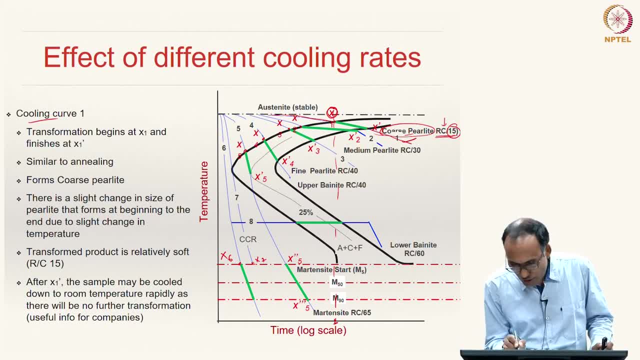 And note that here, when you are cooling down, you can see that at this temperature you are not waiting at constant temperature, you are continues to continuing to reduce, for instance here. So the austenite that has been transformed to pearlite here is happening. 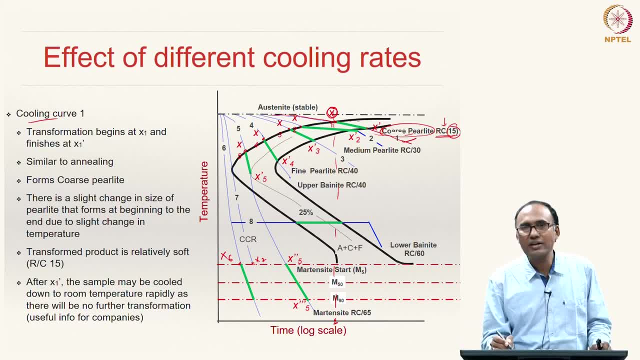 at higher temperature compared to the transformation of austenite to pearlite here at this location. That means here is at lower temperature compared to here, which means the pearlite microstructure is also going to have a gradation. It is coarse pearlite overall but again within that you. 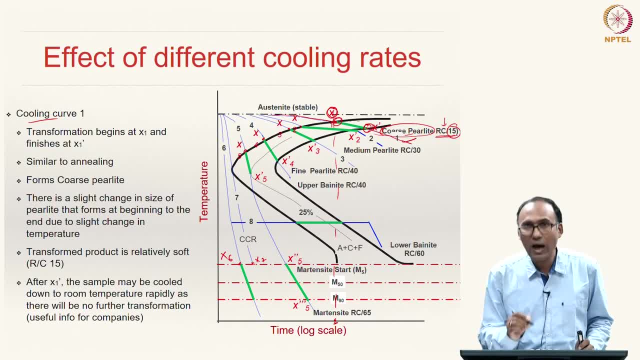 will have the grains of austenite transforming to pearlite. So pearlite here will have a larger size compared to the grains of austenite transforming to pearlite here. So there will be a slight change in the size of pearlite that is forming. 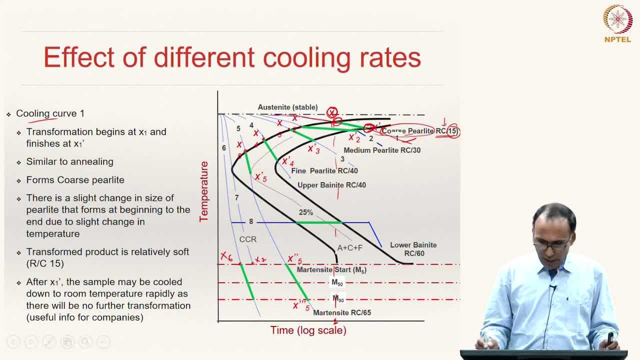 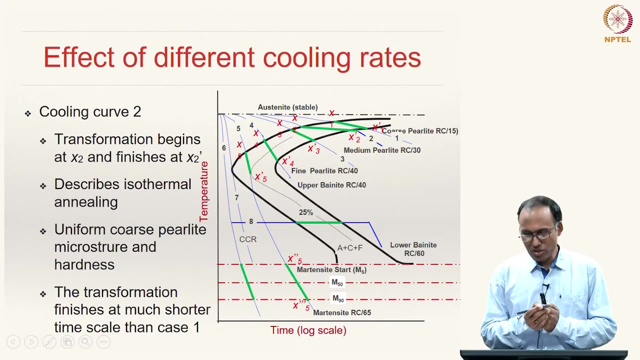 in the beginning and in the end And after x 1 prime. you do not need to wait to continue to cool at the same rate, because all the transformation has happened. Now you can rapidly cool it down. So this sort of an information is going to be extremely useful. 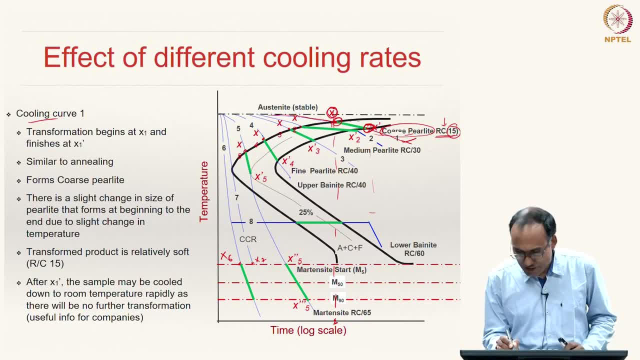 For industry, because you know until what time you need to wait for complete transformation of austenite to pearlite, And after the transformation has happened you can actually cool down at a much faster rate because you do not have to. you do not have any non-equilibrium phases. 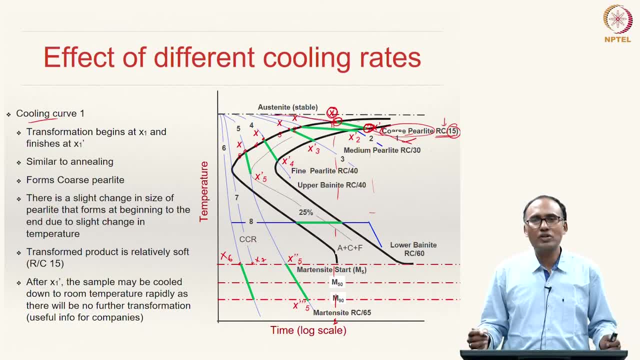 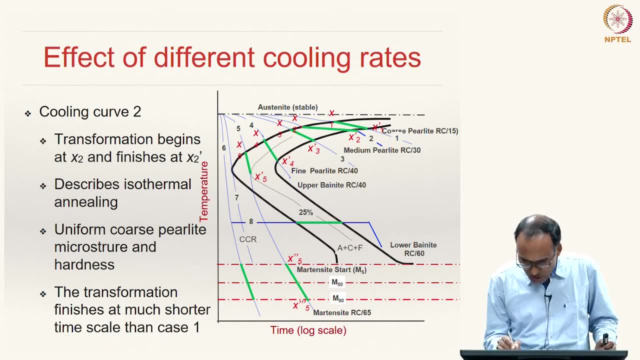 staying there anymore, right? Further cooling down will only reduce the temperature of the component. all right, Now let us look at cooling curve 2.. This is x 2 and this is x 2 prime. So the transformation begins at x 2 and ends at x 2. dash And this: 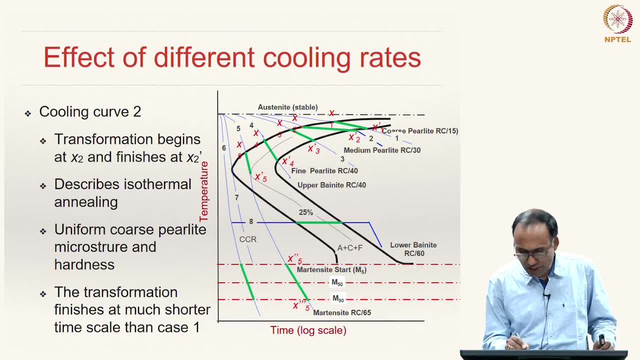 this is sort of represents isothermal transformation. That means you are actually at constant temperature. You are holding the specimen at that temperature And then you can see that you, because it is at constant temperature, the pearlite grain size that you are getting will be uniform. 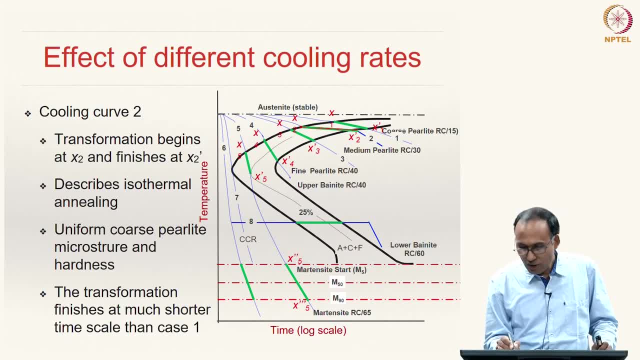 throughout. However, the size of the grain will be smaller than the what has been produced in this region because the temperature here is lower, So you will have a uniform grain. size of the grain will be little smaller than this coarse pearlite, So it is somewhere between: 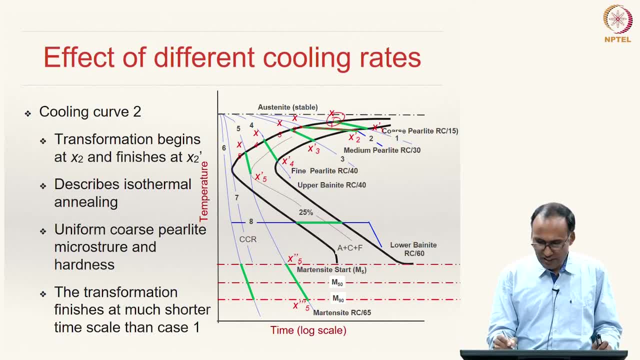 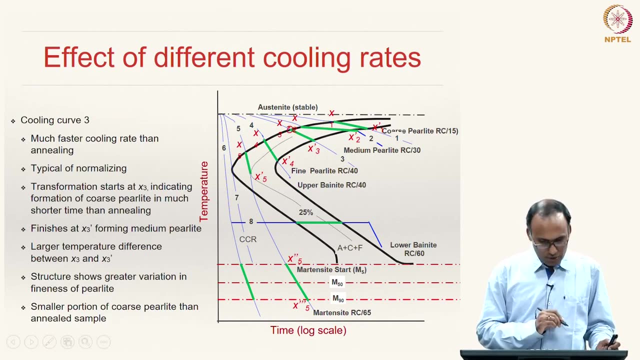 these two sizes and this size and that size, So you will have a uniform coarse pearlite and the transformation finishes at x 2 prime further, after which we can actually cool down rapidly. Now let us look at x 3.. This is x 3.. This is much faster cooling rate and you can see. 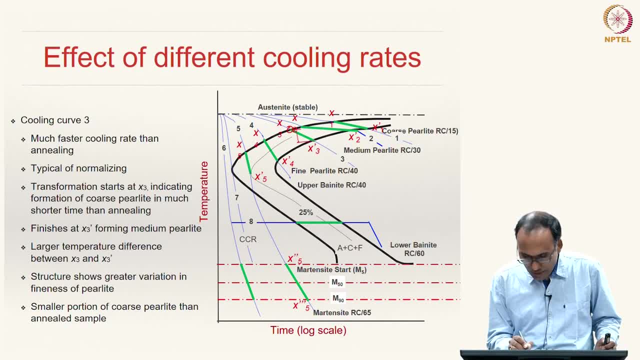 that there is actually the range about which your cooling is actually larger compared to first x 1 prime, x 1 x 1 prime range. So this is typical, So faster cooling rate of this range is typical of a heat treatment process called normalizing. We will see what is normalizing. 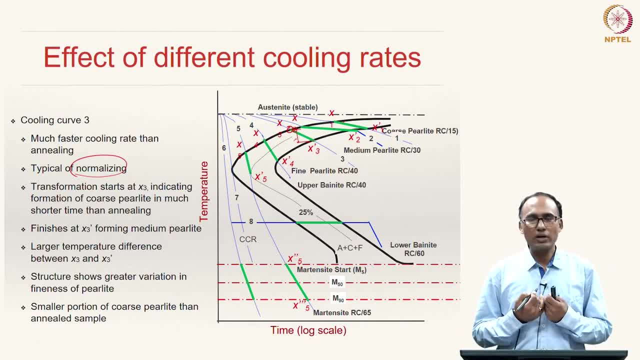 So normalizing uses a higher rate of cooling, whereas the first one where x 1 x 1 dash, that is sort of representing your annealing process. So the transformation begins at x 3. And ends at x 3 prime and you can see that the microstructure of the pearlite is medium. 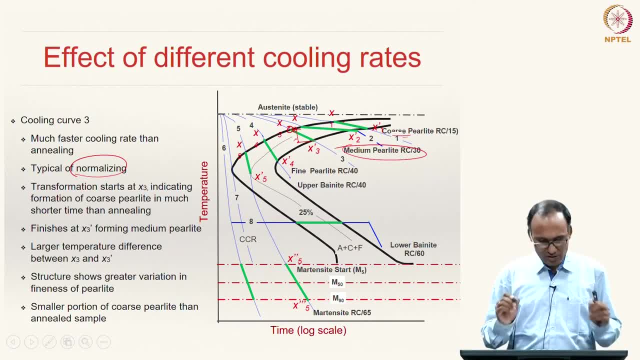 pearlite because it is going to be finer than coarse pearlite. That is why it is called medium pearlite. Again, in this case also, you will have a size variation from the pearlite that is formed in the beginning to the end, So you will have a greater variation in fineness. 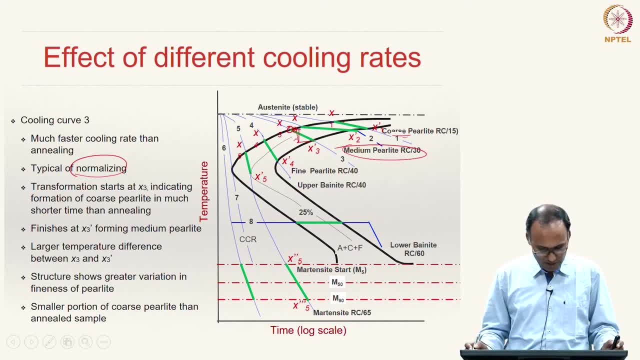 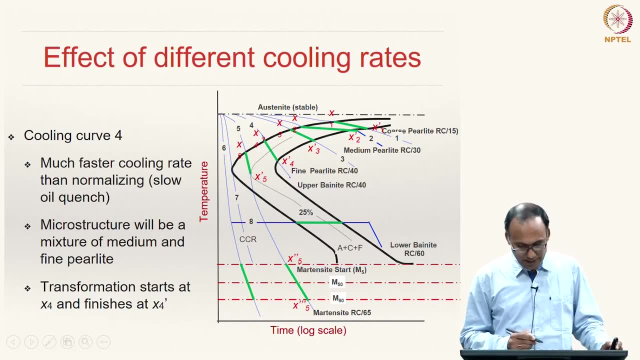 compared to x x 1 prime, because there is a larger temperature gradient. Now let us look at curve 4.. This is x 4. It is much higher cooling rate And you can see that this is very close to slow quenching. 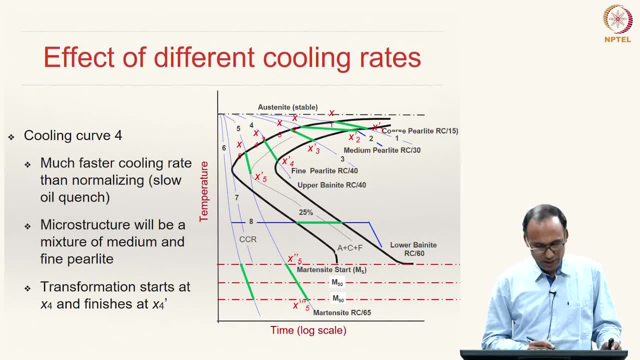 It is not quenching, but it is not very slow cooling rate. So it is also a cooling rate much faster than normalizing. So again, microstructure will be starting from fine pearlite, medium pearlite. So in this region you have medium pearlite, In this region you have fine pearlite. 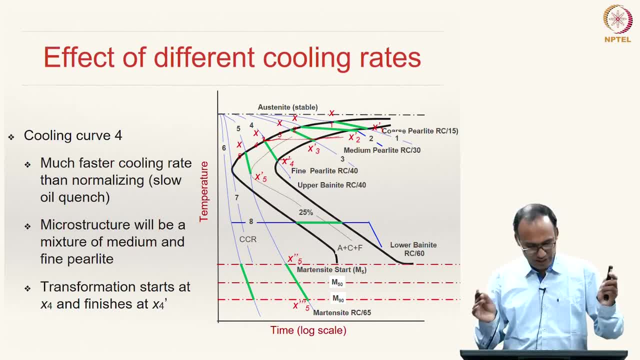 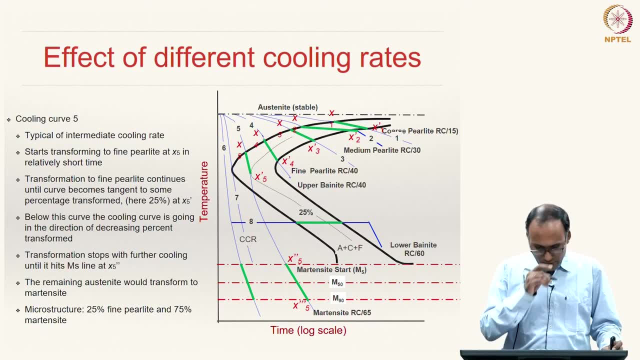 So the microstructure will have a medium pearlite to fine pearlite variation. So you have x 1 prime and y 2 prime And you can see that there is a slightly difference between x 1 prime and x 2 prime. Now, this is the 3 d. 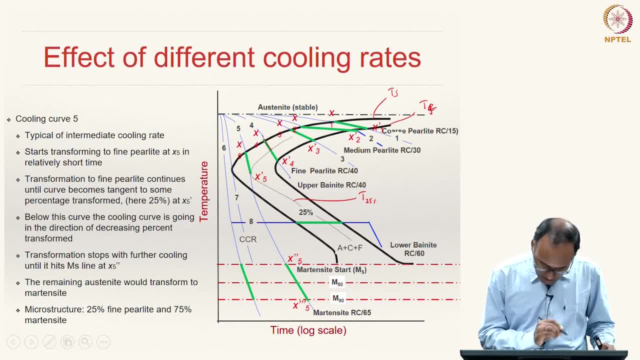 that you have in this region. Now suppose you consider the x 2 prime as the intermediate cooling rate. Perhaps this is the interface of the high temperature, of the high temperature system, which you will find in the 2 d physics. So let us consider the high temperature of. 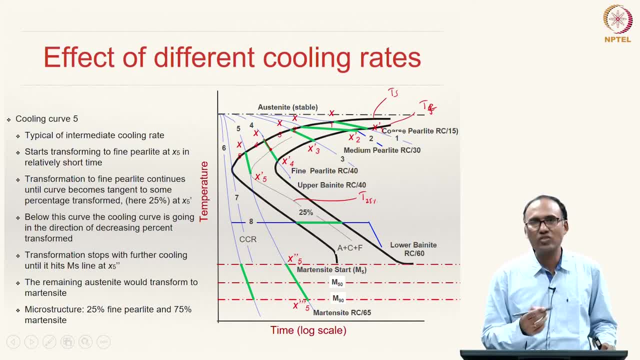 the high temperature system. So as it is getting lower in terms of the high temperature system, it is increasing by 10 to the power of 15.. So you are going to find the high temperature. only 25 percent of your austenite transformed to pearlite. Now, if you come here on the 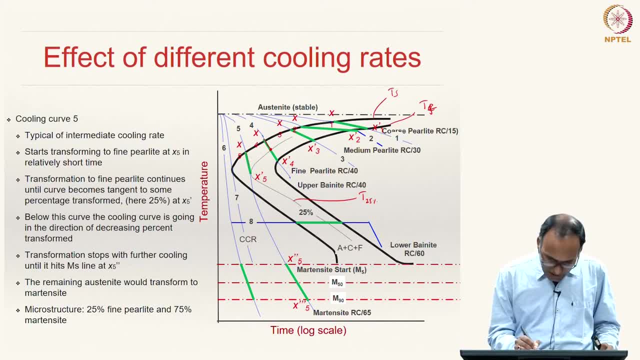 x 5, dash x 5 line. it is becoming tangent to this curve. So suppose, if you are seeing here what will be the transformation, that will be less than 25 percent. That means the moment this cooling curve becomes tangent to one of the transformation fractional lines. 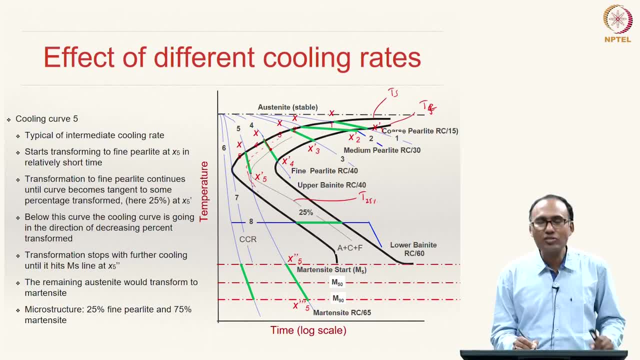 that is when the transformation stops, because below that the transformation is actually less than 25 percent. That means there cannot be any transformation happening and that is the reason why you do not have this green extending throughout this region, only this region. the green is there. So that means transformation happens only from here to here. 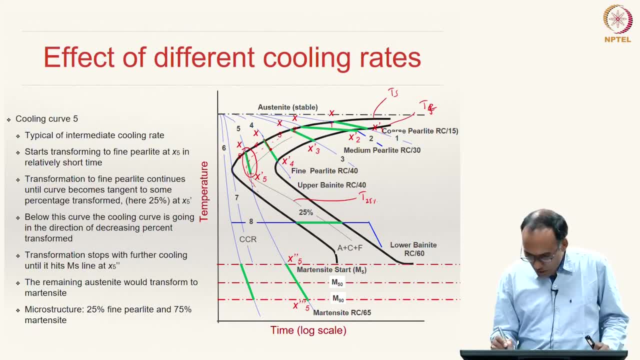 That means what, by the time it reaches here for x 5 to x 5 dash, you have 25 percent pearlite and remaining 75 percent is austenite. You still have 75 percent austenite and you are continuing to cool down at the same rate. 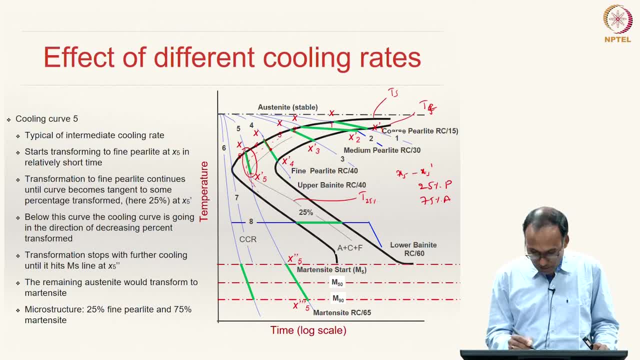 Then you have not have further transformation. and then you have heating martensite start at temperature x, 5, double dash. The moment you have heating martensite start at temperature x 5, dash, double dash, that is when the austenite remaining austenite, 75 percent remaining austenite, will start transform. 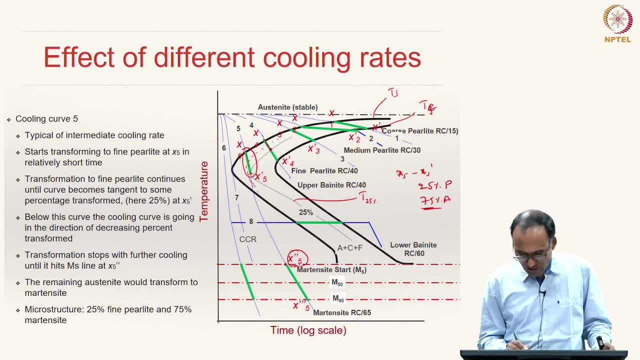 into martensite And martensite transformation. let us say this is finishing, or 90 percent martensite is transform or we will. in this case we will. let us assume that it is finished temperature. then the remaining 75 percent austenite would have transformed to martensite. So here the 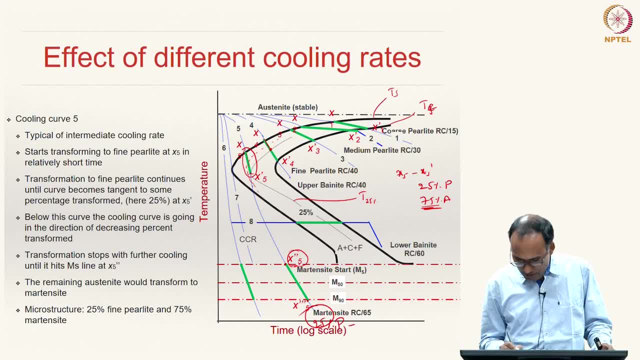 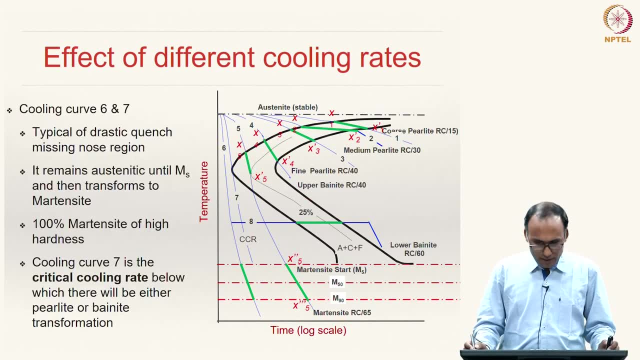 microstructure will be 25 percent pearlite plus 75 percent martensite. That will be the microstructure. And now let us look at X 6 and 7.. If you see X 6 curve, for instance, let us look at. 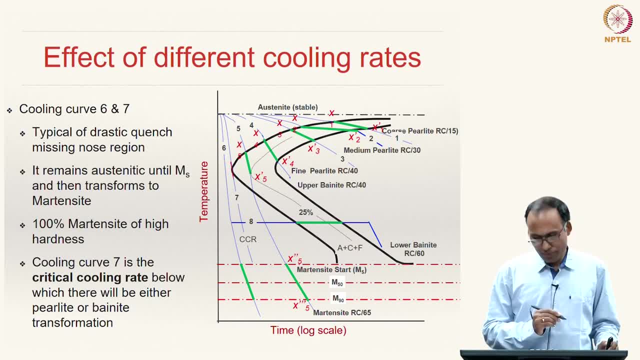 X 7. first, It is actually tangent to your martensite, sorry, the transformation start line. That means it is never going into the two-phase region. That means there is no transformation of austenite to pearlite that can take place. So this rate of cooling is: 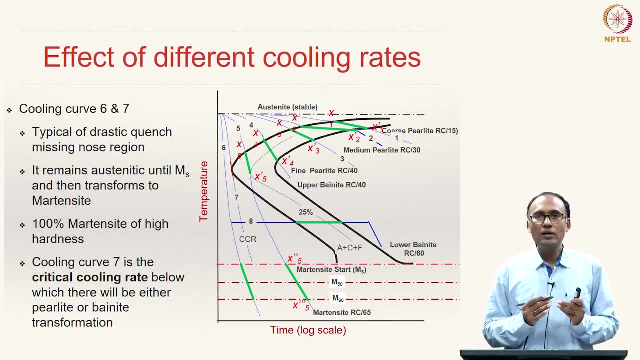 what we call a critical cooling rate, The cooling rate below which only the austenite to pearlite or bainite transformation takes place, above which the austenite will not transform to either pearlite or bainite: It will directly transform to martensite. So 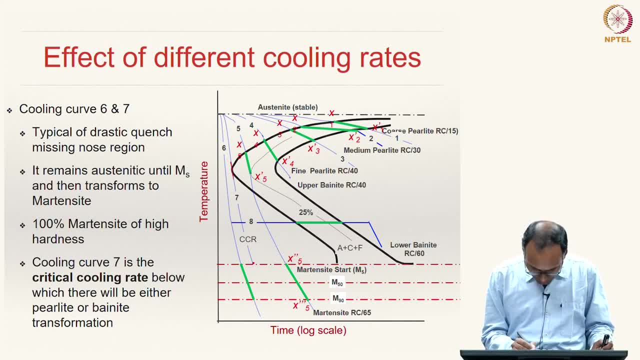 you can see austenite. this 7, cooling curve 7 ends here. actually, If it is ending here, what happens At this temperature? you have stopped. That means you are not further reducing the temperature. So all the microstructure will be only of austenite because you have 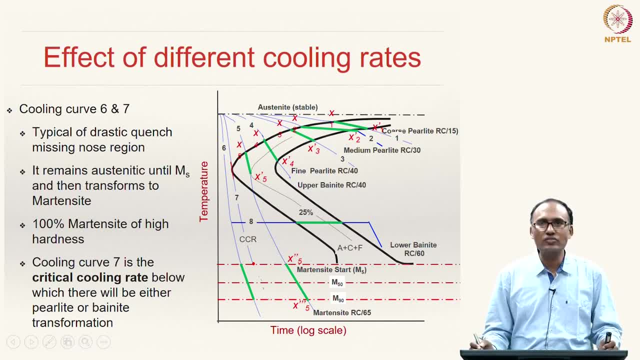 not transformed further. You have not reduced the temperature further because the martensite transformation requires you to go below the…. You continue to reduce the temperature. If you do not reduce the temperature, even if you wait there for sufficiently long time, the no transformation takes place. Now look at the 6.. So 6 continues to cool. 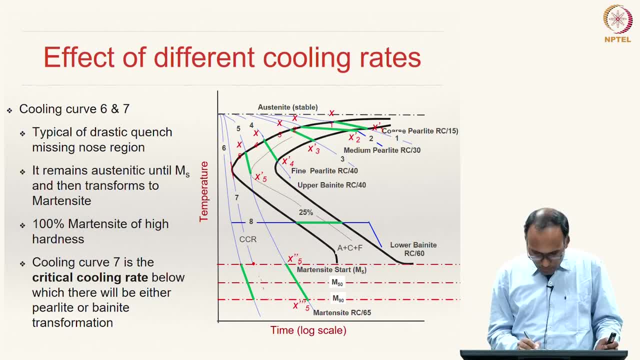 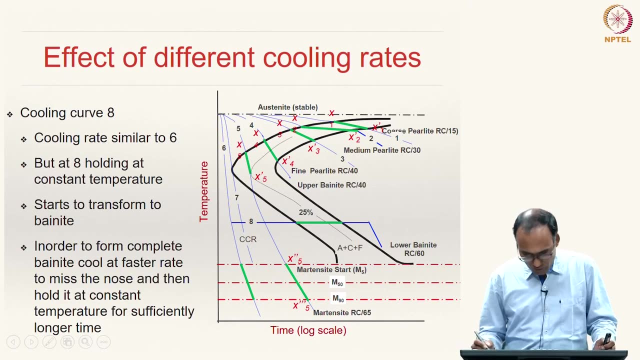 down. So here it is continuing to cool down. That is when all austenite is transforming to martensite. So here microstructure will be 100 percent martensite. And let us look at cooling curve 8.. So how does this look like? So you can see that. 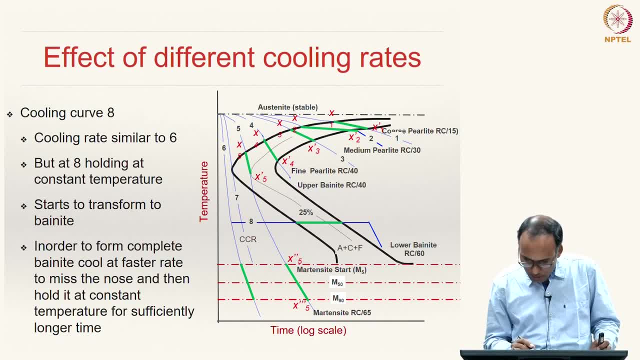 right. You can see here it is very high cooling rate, but you are not continuing to cooling down, You are holding at this temperature And this temperature is your below the nose. The moment you are coming below the nose, all the austenite will have to transform to. 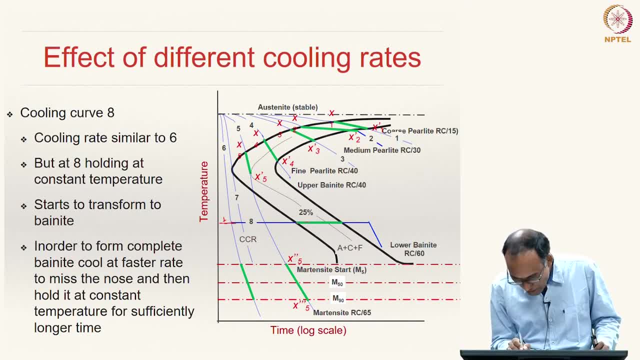 bayonet, right. So that is why you see that this is all transforming to bayonet. So the microstructure here will be 100 percent bayonet. This is basically a medium here. very close to nose will be upper bayonet, far away from the nose will be lower bayonet. So it is somewhere. 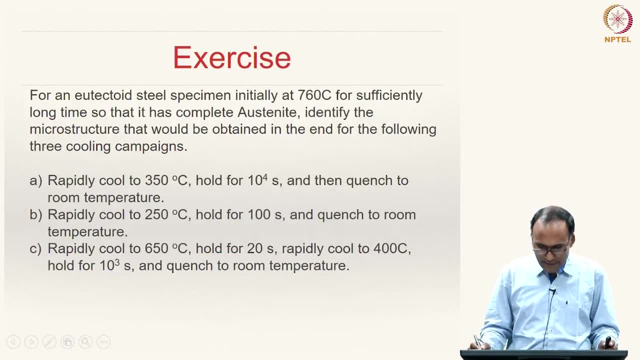 close to lower bayonet. all right. So now let us look at by learning how this cooling curves work. Let us try to solve this problem for a detector steel specimen, initially at 700 degree Celsius, 760 degree Celsius, for sufficiently long time so that it has complete austenite, So it is completely austenitized. 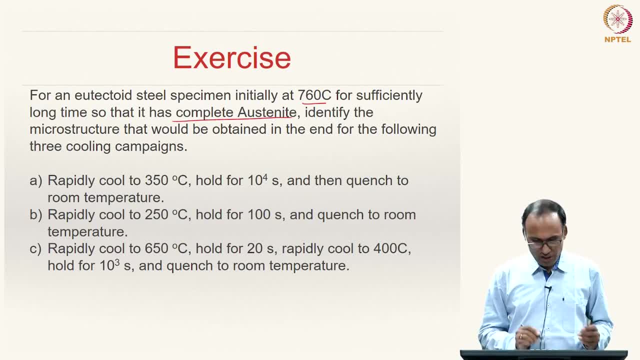 Now, if it is in complete, all the microstructure is austenite. Now identify the microstructure that would be obtained in the end for the following 3 cooling campaigns. So first one is: if you take this guy and rapidly cool to 350 degree Celsius, He has hold for 10 power 4 seconds. 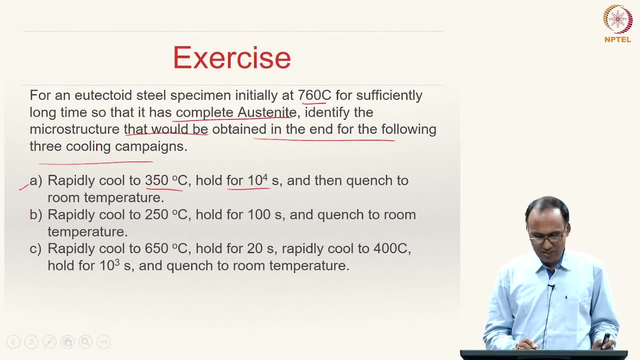 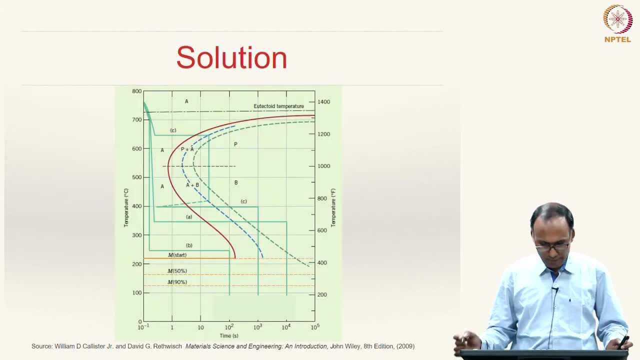 Let us look one after the other: Rapidly cool to 350 degree Celsius and hold for 10 power, 4 seconds, and then quench to room temperature. So here you have these cooling lines drawn: Rapidly cool to 350 degree Celsius and then. 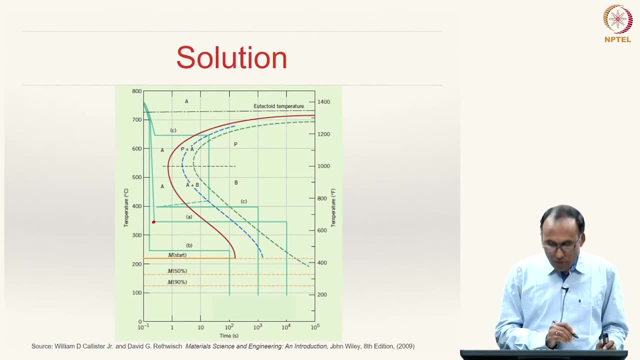 So that is this guy and then wait for there for 10 power 4 seconds. So you are waiting there for 10 power 4 seconds. So you are actually missing the nose. since you have missed the nose, the transformation. it is above the martensite start temperature. So here still. 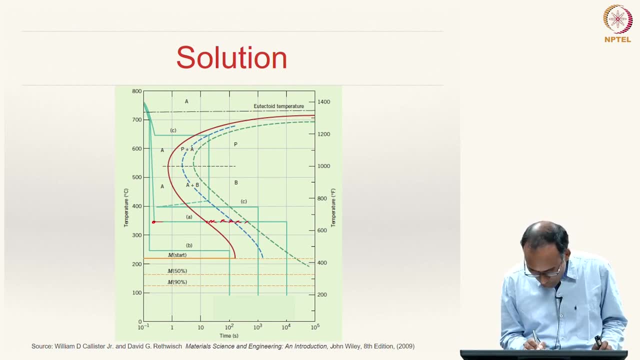 bainite can form. So during this process, by the time it comes here the bainite would have austenite, would have transformed to 100 percent bainite, So you will have completely here the microstructure will be 100 percent bainite. So for the case A, you will have. 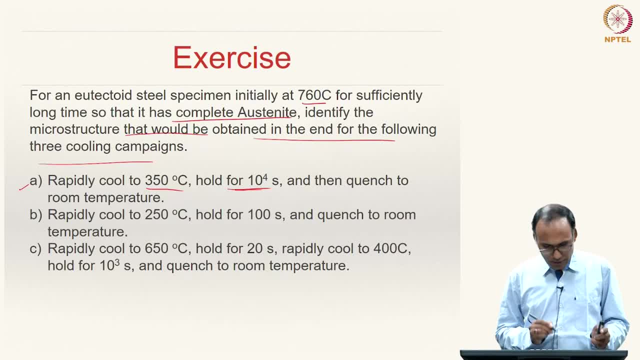 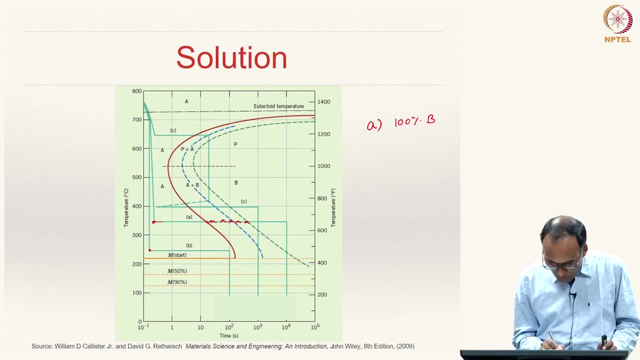 100 percent bainite and for case B, rapidly cool to 250 degree Celsius, hold for 100 seconds and then quench to room temperature. right, rapidly cool to 250 degree Celsius. that is 250 degree Celsius, and then hold for 100 seconds. 100 seconds is this, and then I am holding. 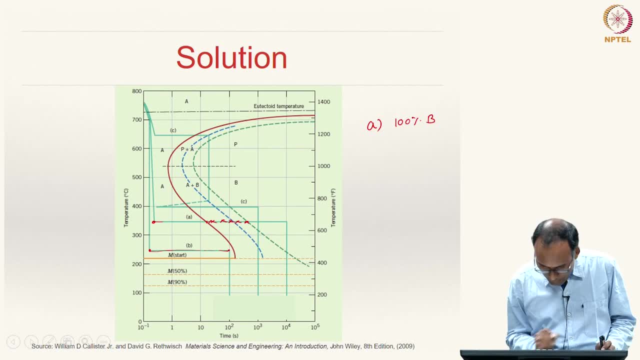 for I came below the nose and I am holding here for 100 percent bainite. Even after holding for 100 seconds, we did not hit the transformation, the start line, this red line, and hence nose. transformation of austenite to ferrite takes place- austenite. 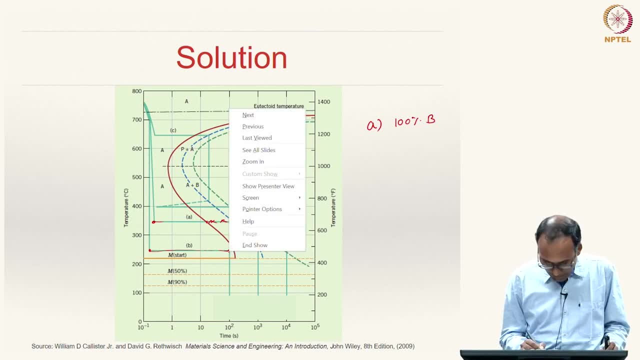 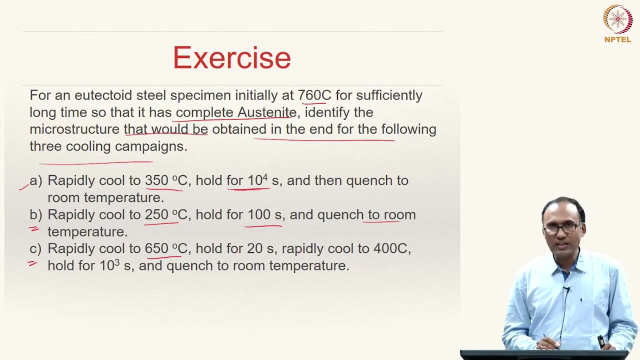 to bainite takes place, but then we are quenching it down, and hence what should happen here: all the austenite will be transforming to martensite, So that will be 100 percent martensite and the case C rapidly cool to 650 degree Celsius, hold for 20 seconds and then quench. 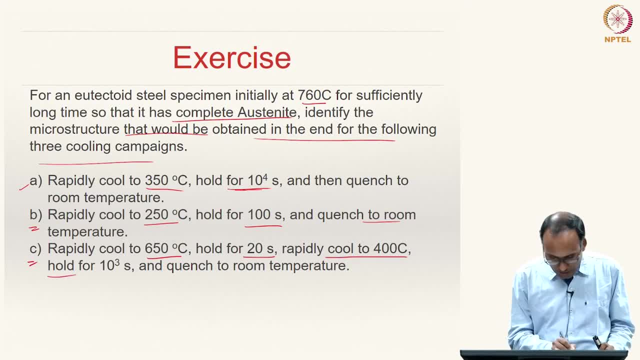 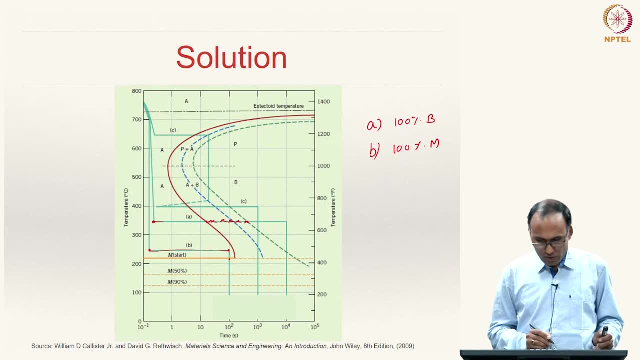 And then rapidly cool to 400 degree Celsius and hold for 1000 seconds and then quench to room temperature, right? So first rapidly cool to 650 degree Celsius and there hold for 20 seconds. So this is 10, so 20 is somewhere here. So we are holding for 20 seconds. that. 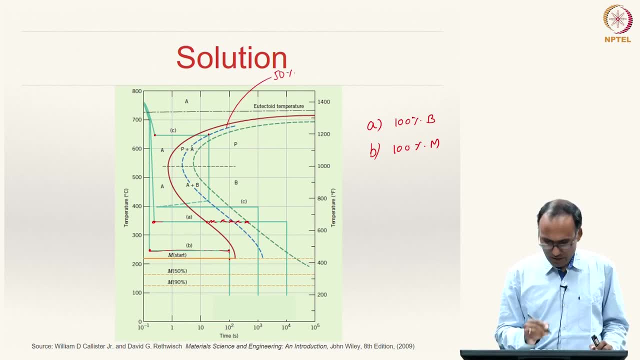 means it is. if it is not written, that means it is 50 percent line. if nothing is written here, right, whether it is 25 percent or 50 percent. if it is not written, then it means it is 50 percent line. So what happens here? austenite transforms to. by the time, here in the C, austenite is transforming. 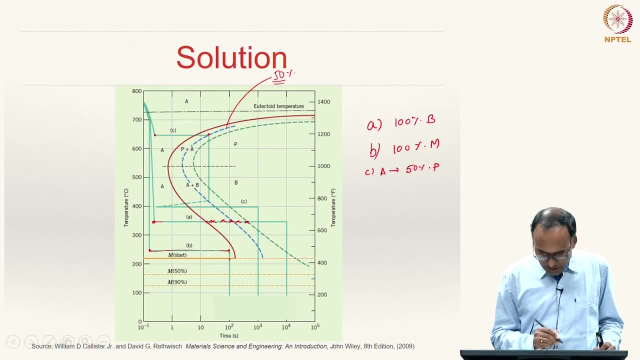 to 50 percent pearlite. is it fine pearlite or coarse pearlite? here you have coarse pearlite, So it is 50 percent coarse pearlite. microstructure is coarse And then you are suddenly cooling it down because now you are not allowing it to go. 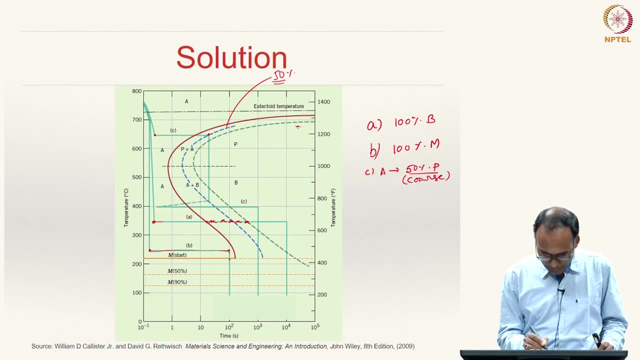 continue. So you are not allowing it down. only 50 percent of it is converted to pearlite and you are continuing cooling down at 400 to 400 degree Celsius, and then your time starts again, right? that is why this dashed line, just to show that your time starts again and again. you. 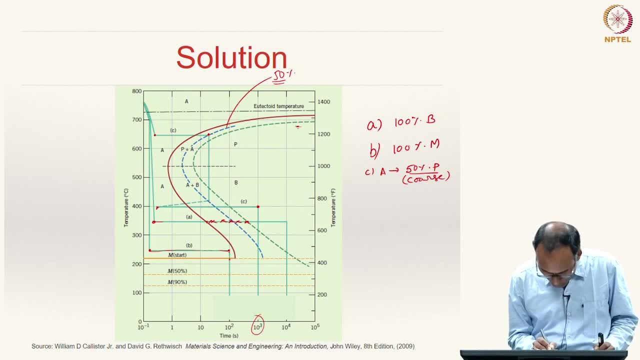 are waiting for 1000 seconds. this is 1000 seconds and you are waited here. So what happens? because you are now, by the time you are quenching. you are actually going below the nose here and hence, as a result, you will be the remaining austenite if at 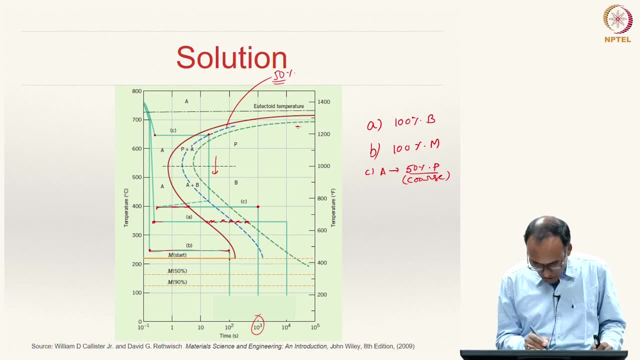 all hits. it is hitting the transformation start line. So the remaining 50 percent austenite. So the remaining 50 percent austenite. So you have 50 percent austenite and 50 percent pearlite by the time. 50 percent austenite- 50. 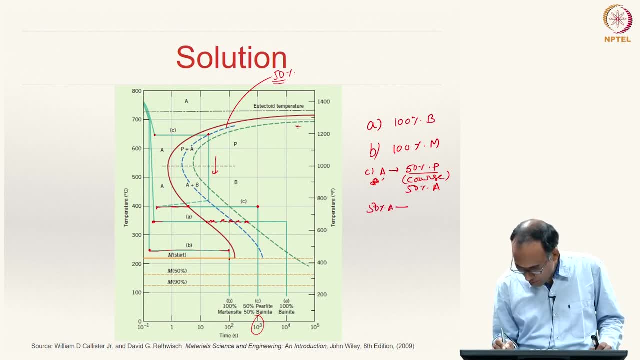 percent pearlite. So the remaining 50 percent austenite will convert to the 50 percent bainite total. So here all the austenite, all the remaining austenite will convert right. all the remaining austenite is converting means it is 100 percent is converted what is actually available out. 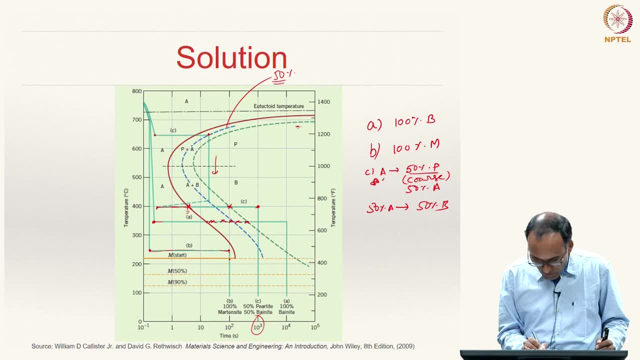 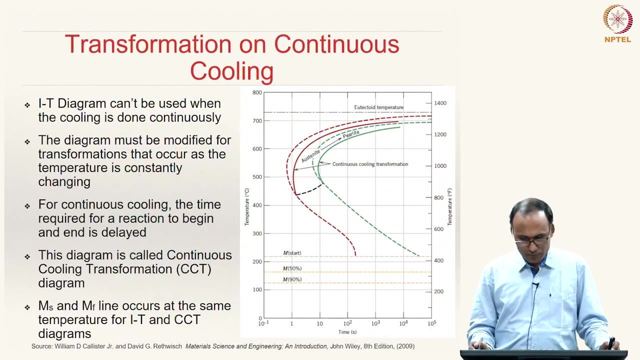 of the original composition only 50 percent is available, So that whole 50 percent is converted to bainite. So you can see that the third one has 50 percent pearlite and 50 percent bainite, right? So that is about the isothermal transformation. 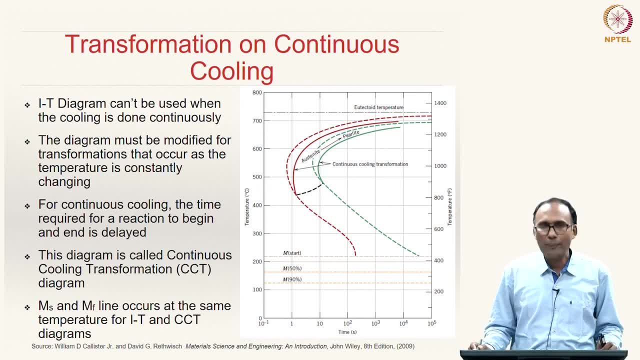 But now let us actually look at what happens when you are continuously cooling, because the continuous cooling is something that would happen in the industry, not usually the isothermal transformation. that is why the continuous cooling is very important. So the transformation on continuous cooling is something that we would look at. So the I-T diagram in isothermal transformation: 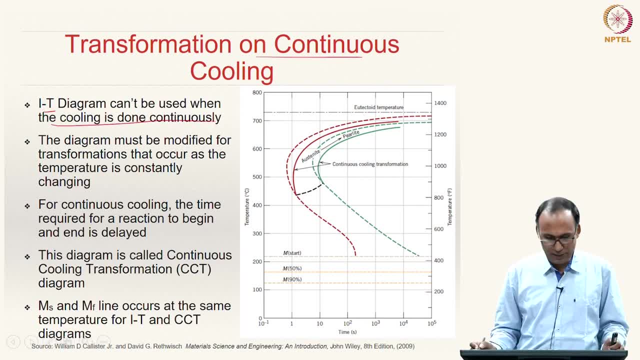 diagram cannot be used when the cooling is done continuously, And hence you need to modify the diagram for transformations that occur as the temperature is constantly changing. So what happens is so this here, the dashed lines, represents your isothermal transformation diagrams, and then the because if you are doing continuous cooling, then your start martens. 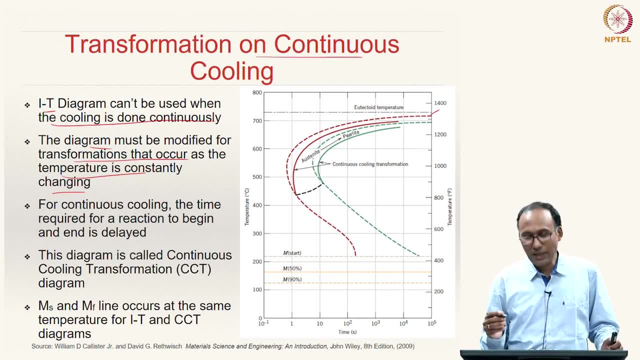 sorry. the transformation start time and the martens transformation end times are going to increase as well as the temperatures are going to reduce. So for a continuous cooling the time required for reaction to begin and end are delayed And the diagram is called T-T, C-C-T diagram, that is, continuous cooling transformation diagram as opposed to T-T-T. 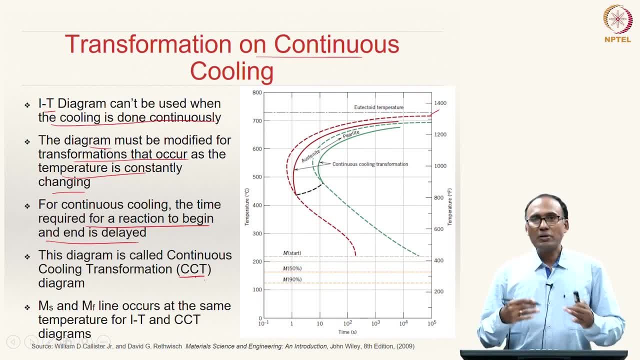 diagram Here. because we are doing continuous cooling, these two curves change, but the martensite start and martensite finish temperatures will not change because they do not depend on the cooling rate. So because of this fact, for our eutectoid steels, you can see that because 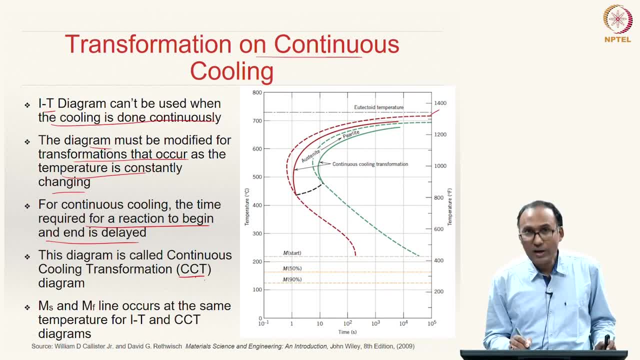 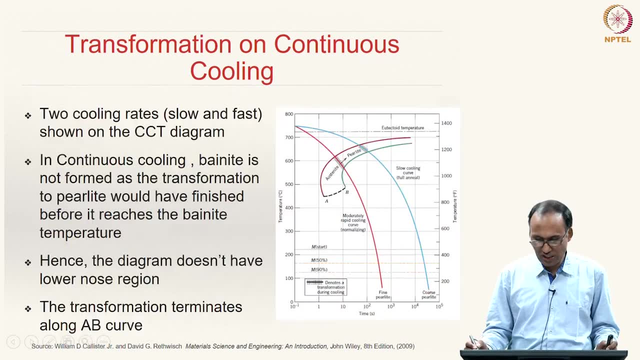 you are. if you are doing continuous cooling, you will see that you will not have the nose region below the nose region, So your transformation finishes above the nose region itself, right? So here you have two cooling regions, Bless. Now let us make the DANIEL standard image so you can see all the left and right You. 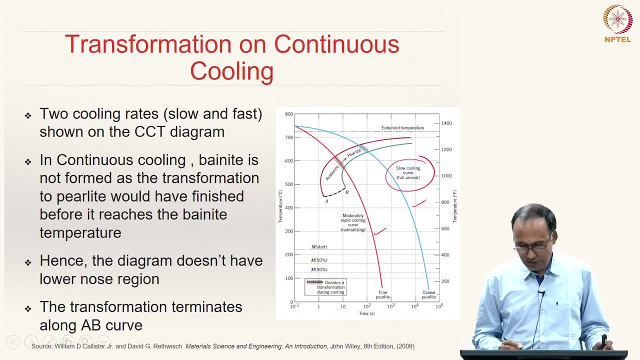 can see all the left and right And if you repeat the previous, the same, It will change. this shown Here. they are some of the two curves. These are discussed here. These are two cooling rates. Hello, I am Sylee. briefly name is Ali. this is Slye. 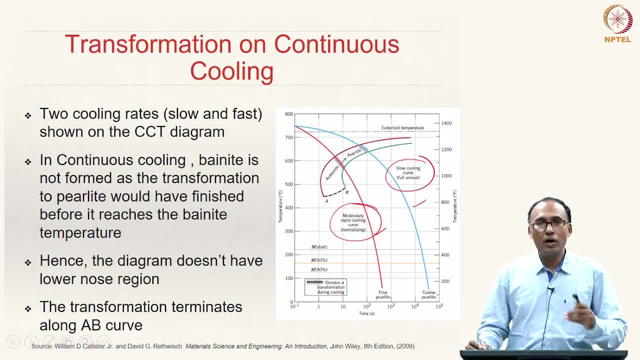 I want to show you. the first wave here is quite simple. the- the first curve is judicial cooling. It will differ. there are different forb, Просто one rate. They are far, each time currents. it will be like the length of the curve, the procedure. 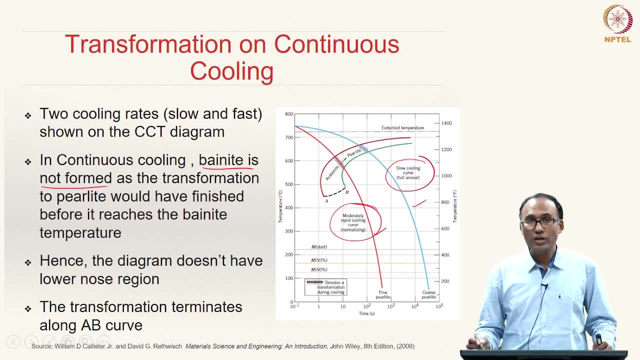 is performed Where 1.cE, 2.d- b4-3.d-3, when you are dealing with eutectoid steels, as the transformation to pearlite would have finished before it reaches the bainite temperature because you are continuously cooling. So 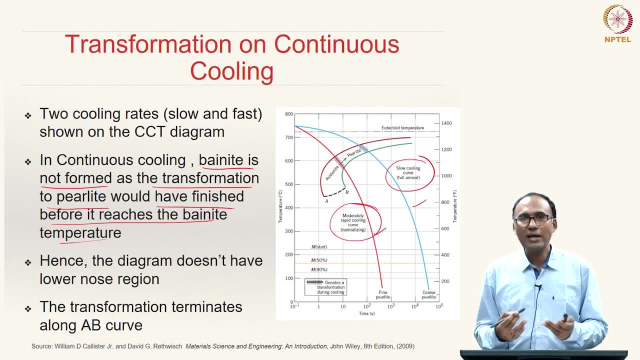 you would always finish your transformation by the time you hit the nose. So by the time you hit the nose, all the austenite has already transformed to pearlite, and hence there is no possibility for transformation of bainite in the case of continuous cooling in eutectoid. 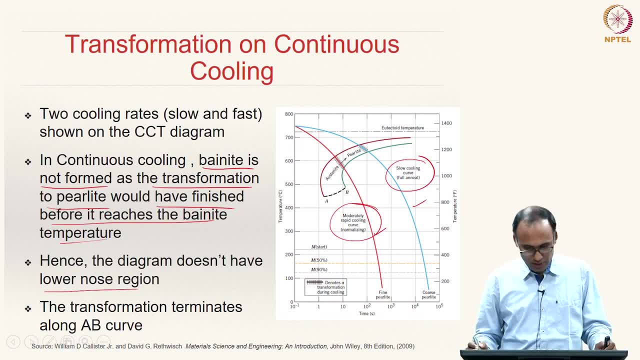 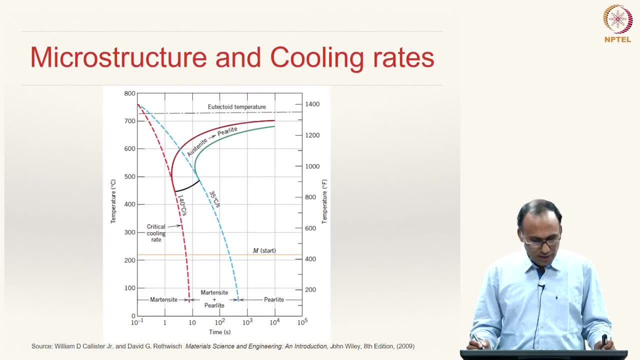 steels. So that is why diagram does not have lower nose region and the line AB. the transformation terminates along the line AB. So we know that the cooling rate is called critical cooling rate when there is no transformation of austenite to pearlite. but all that means it basically misses the nose. then you can. 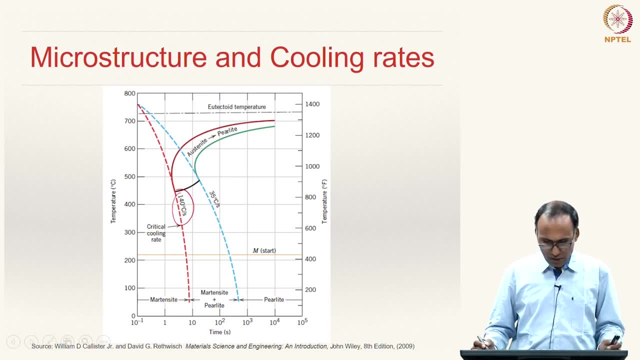 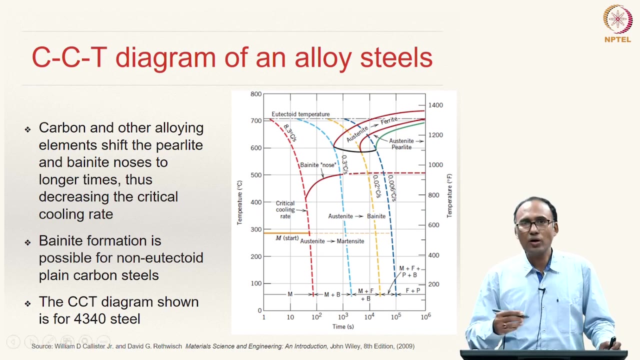 see that this 140 degree Celsius is cooling rate, represents your critical cooling rate. So all right. And however, for an alloy steel, which is a more complex steel than a eutectoid steel, you can see the nose region, So the bainite formation is possible for alloy steels. 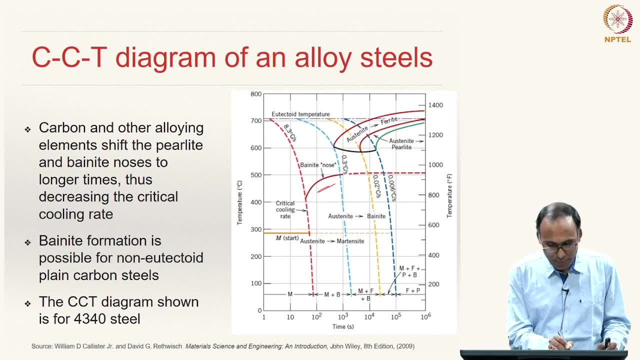 but not for eutectoid steel, as we have seen before The carbon and other alloying elements. what they do is they shift the pearlite and bainite noses to longer times and thus decreasing the critical cooling rate. So bainite formation is possible for non-eutectoid plain carbon steels. It is possible Only. 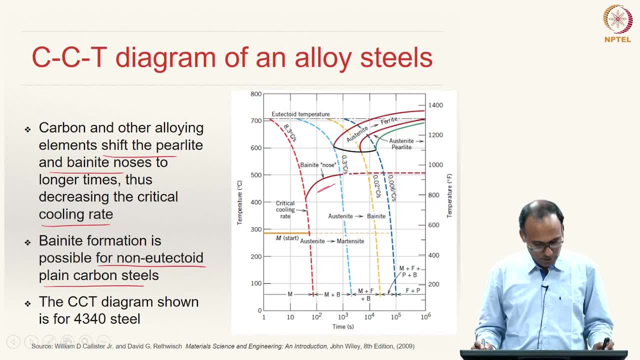 for eutectoid steels. you can see, you see that it is not at all possible. So this is the CCT diagram: continuous cooling transformation diagram shown for 4340 steel, whereas before we have seen the time temperature transformation diagram for the same steel, So for different. 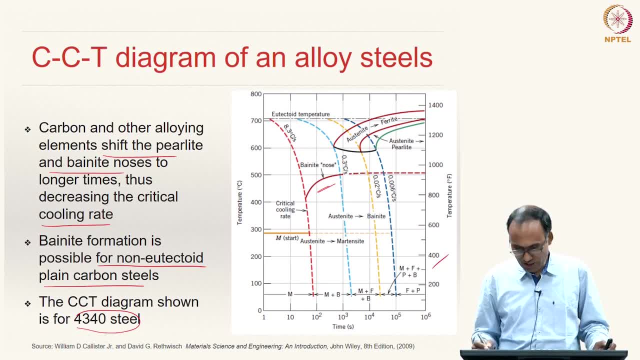 cooling rates, one would be able to find out what is the microstructure. Here we have shown different cooling rates. The critical cooling rate is given here. So here we have shown different cooling rates. So here we have shown different cooling rates. The critical. 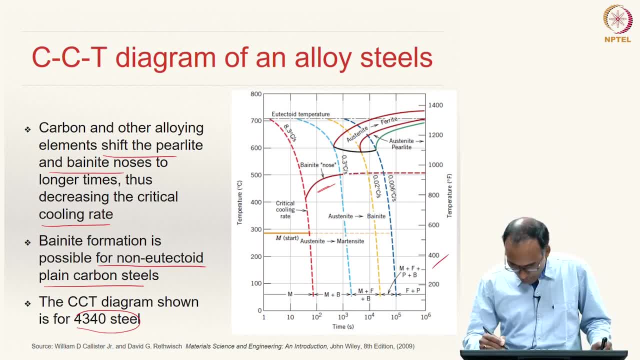 sort of boundary cooling rates. For instance, if your cooling rate is between this blue line and the orange line, you will always form this such a microstructure- martensite plus ferrite, plus pearlite plus bainite, because you will have this austenite to proeutectoid.